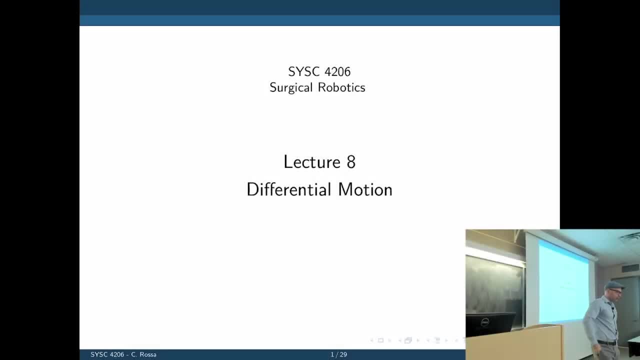 Today we have a lecture on differential motion. We did forward inverse kinematics and what we are doing there was to relate position from the actuators to the position of the robot's tip, Rotation angles to Cartesian position and orientation, or displacement of prismatic joints to Cartesian position and orientation. What about speed? How does the speed of a given 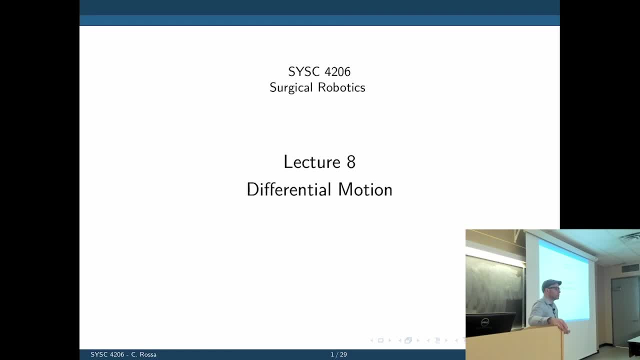 joint affect: the speed of the end factor of the robot. That's what we're going to see today. Why is that important? Well, let's assume that you want the robot to be positioned in a specific orientation in the body, and then you want the robot at that specific orientation to be able. 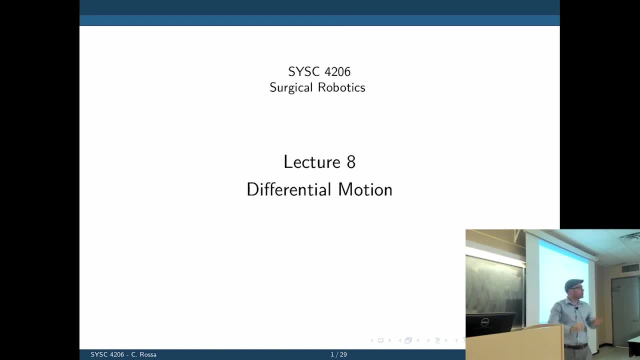 to move in all possible directions, But that is not necessarily the case. There could be configurations- You probably heard the word singularity before. Alec probably mentioned that. Those are configurations of the robot arm in which the robot cannot move in a particular direction. 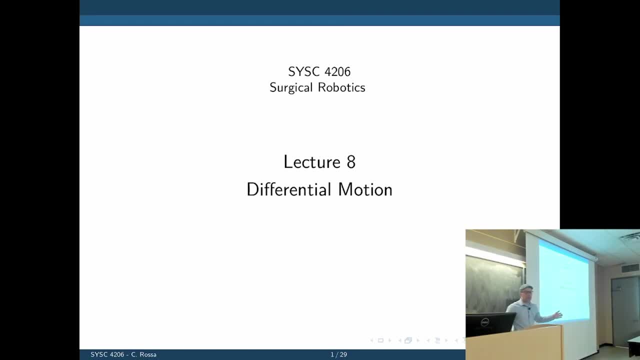 And you can see that through the analysis of differential motion you're going to see today. So basically now shifting the focus from position to position, to speed, to speed and then later torque and force. So the objective of the lecture is to study the concept of Jacobian, which is 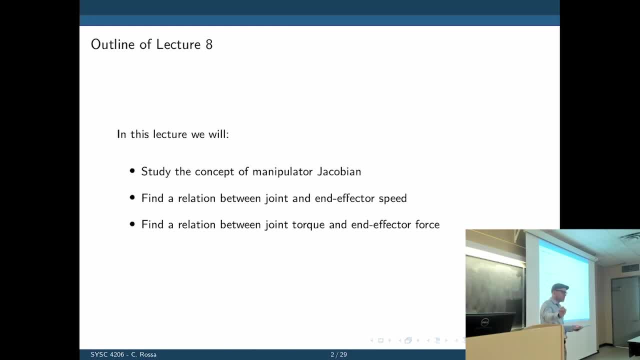 exactly that: a relation between actuation and position. So we're going to look at the concept of Jacobian, which is exactly that: a relation between actuation and position. Speed and Cartesian speed of the robot. Find the relation between the joint and end factor of speed and the relation 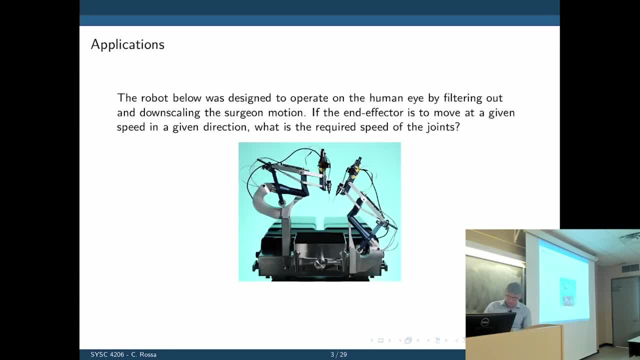 between joint torque and end factor force. Here's an example. The robot below was designed to operate in the human eye by filtering out a downscaling the surgeon's motion. If the end factor is to move at a given speed in a given direction, what? 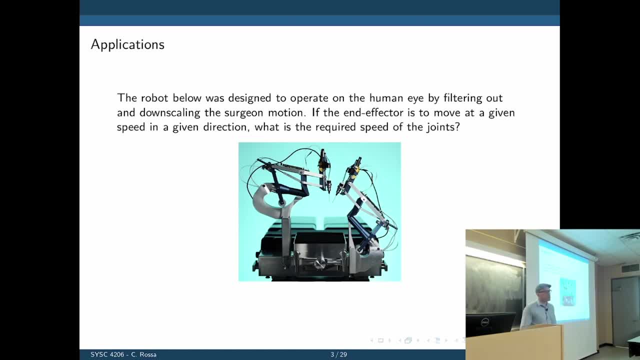 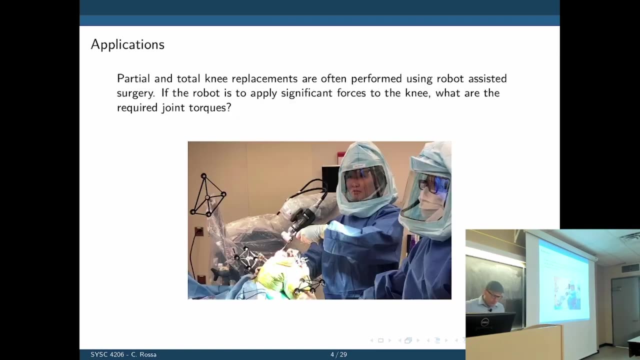 are the required speeds of each joint. Now we know how to do that. for position, Is the speed the same? Well, not quite. Here's another example. Partial and total knee replacements are often performed using robot assisted surgery. If the robot is to apply a 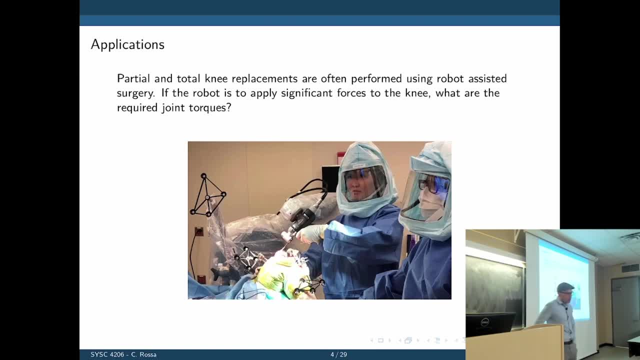 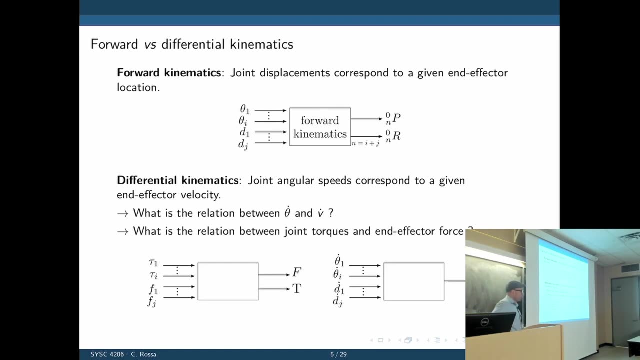 significant force to the knee. what are the required joint torques? In other words, how do you control the direction and magnitude of the force at the tip of the robot by controlling the torque provided to individual actuators. Let's get right into it. We studied the forward kinematics and the forward 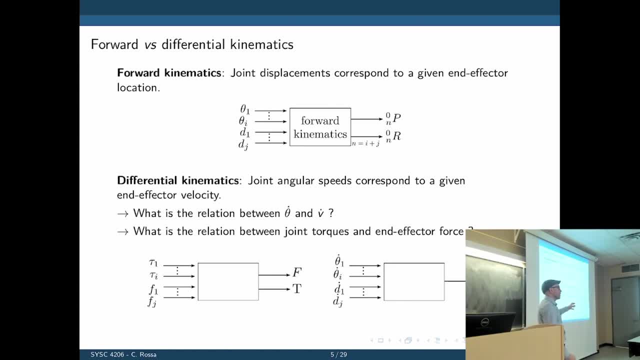 kinematics was the relation between position and position. It's a simple function that you can get from the homogeneous transformation matrices. We input all the variables that we have control of and the output is the position and orientation of the tooltip or the position of an orientation of. 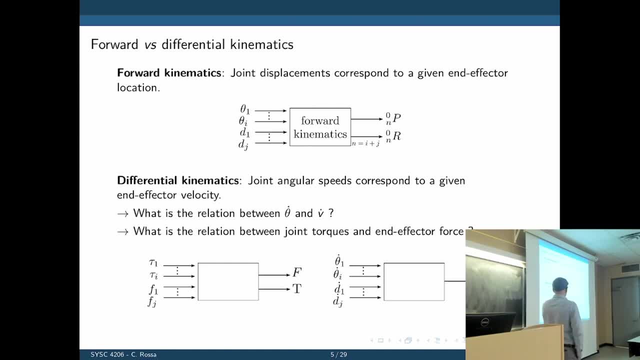 any point in the robot arm, any point in the robot body. The differential kinematics is some sort of similar analysis, but now we are relating joint angular speeds to the position, the speed of the end-effector. So if you call here the position of the joints theta and the position of the prismatic joints d theta, 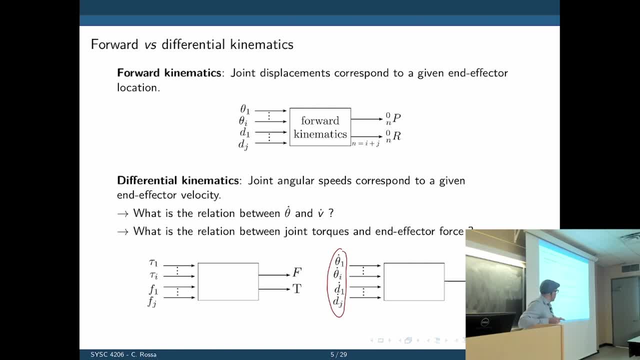 dot and the prismatic joints d dot. the output will now be the time derivative of the homogeneous transformation. to some extent, We can also use what you're going to see today to relate now the torques and forces applied by prismatic or revolute joints. 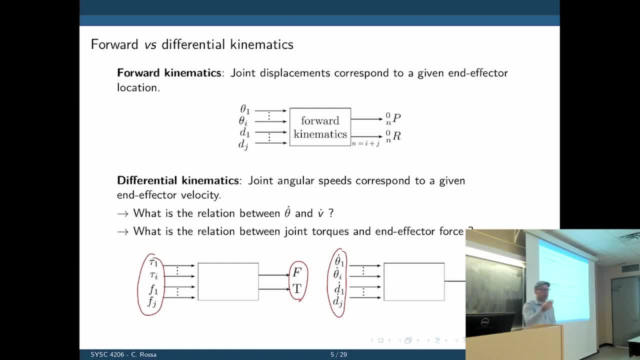 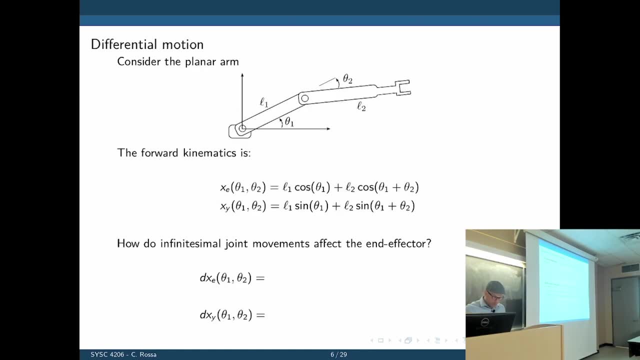 to the force and torque applied by the robots and the factor on its environment. All right, so let's do an example. Let's just start with an example. that's probably the easiest way. We have this two DoF planar arm with two revolute. 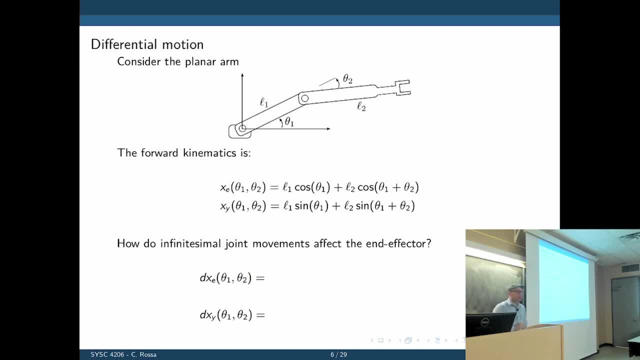 joints and we have the forward kinematics that we calculated before for that robot arm. It depends on theta 1 and theta 2 that you can see- here is one, here is the other one- and on the length of each arm. So if you want to relate, 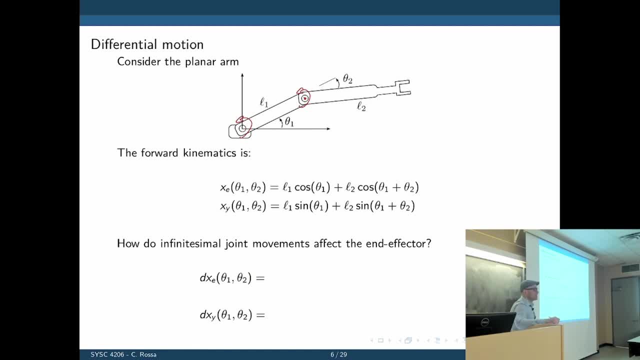 position to position. we know how to do that. Now, if you want to relate speed, then you're talking about a differential amount of position change, a small change in position which over time, would characterize the speed. So if we apply a 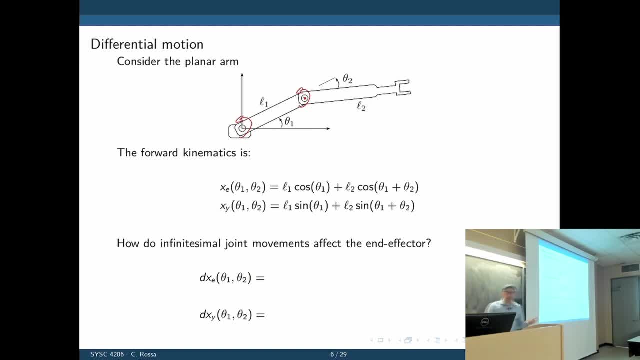 very small change in position. how does that affect the? what change in position does it create? at the tools and the factor? You would say: well, that's simple. just take the derivative of the forward kinematics with respect to all degrees of freedom, that is, theta 1 and theta 2, because those are the two that 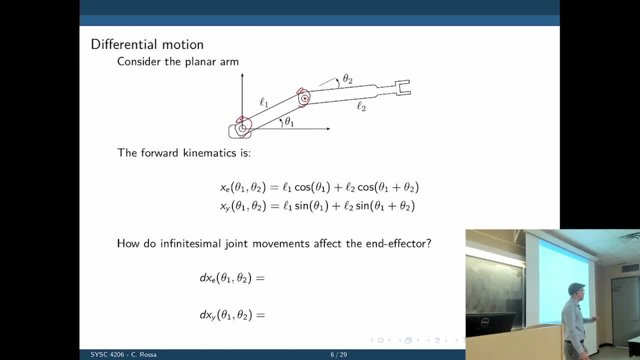 can change the position of the factor. So if you take the derivative of this equation with respect to theta 1 and theta 2, then there we have it, our first insight into how these relations would occur. But before we go and take the 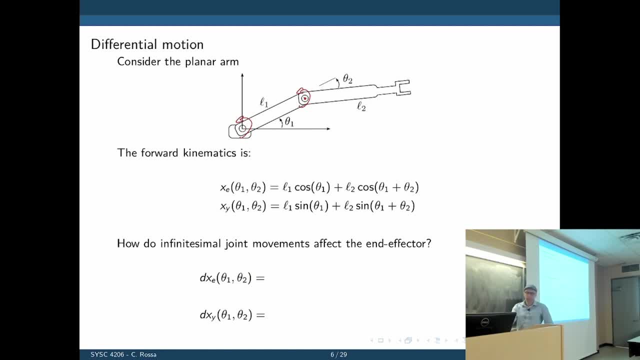 derivative of this expression. let's just do a example. So let's take the derivative of this expression. let's just do a generic derivative that now takes a small change in displacement. Let's call that a small displacement d theta. Now we're applying a d theta 1 and d. 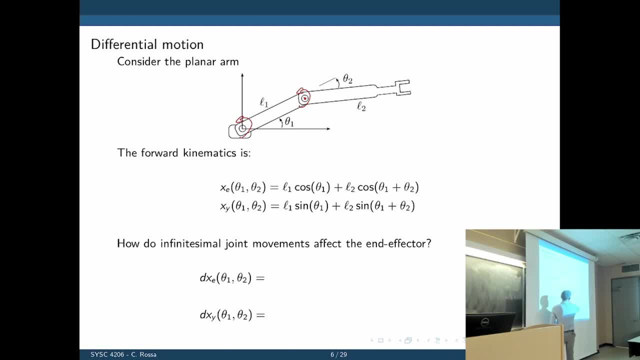 theta 2 to each of joint, which is equivalent to now calculating the effect of that small theta on xe and xy, which is the position of the robots and the factor. Let's consider first the x, the change in position in the x direction, If you. 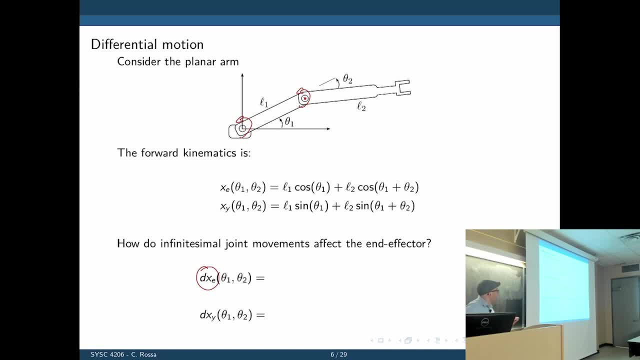 apply a small. if you take a derivative with respect to theta 1,, if you take the derivative of this with respect to theta 1, we are simply doing the partial derivative of ex with respect to theta 1.. All right, chain rule. what comes next? Derivative of x d theta times, times d theta 1.. 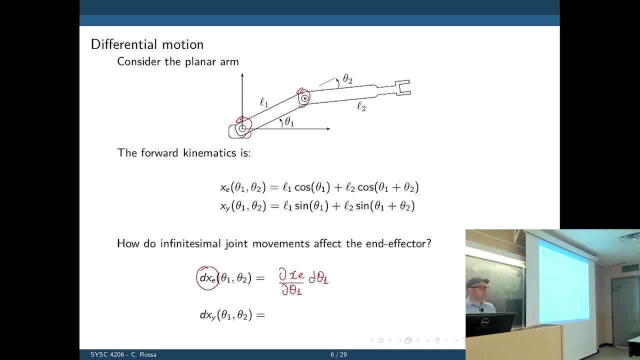 All right, that's the chain rule. Well, that's not all, because we also have now the, the effect that is generated by changing theta 2.. So if you do them both at the same time, then you need to change theta 2.. So if you do them both at the same time, then you need to change theta 2.. So if you do them both at the same time, then you need to. 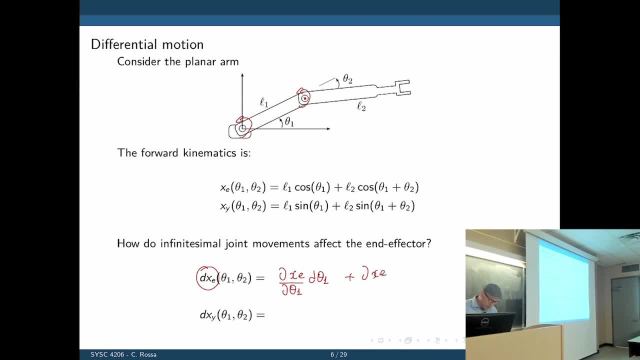 add the partial derivative of x with respect to theta 2, d, theta 2.. So are we saying here I'm applying a small delta, theta 1 and 2, and analyzing the effect it creates in the Cartesian position in the x direction. What's the? 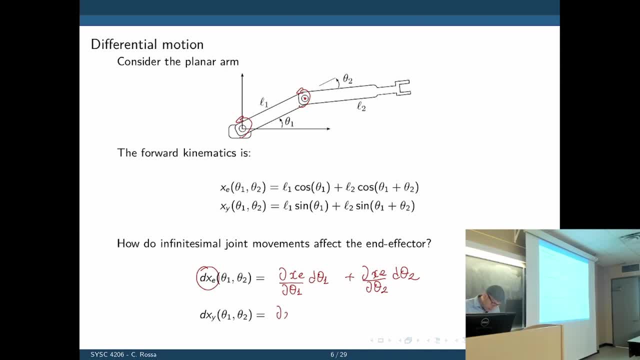 other one. Well, the other one is identical, but now we do that in the y direction. All right, then you add them up to find the final, final relation. So I have it here. these are the same equations on top. 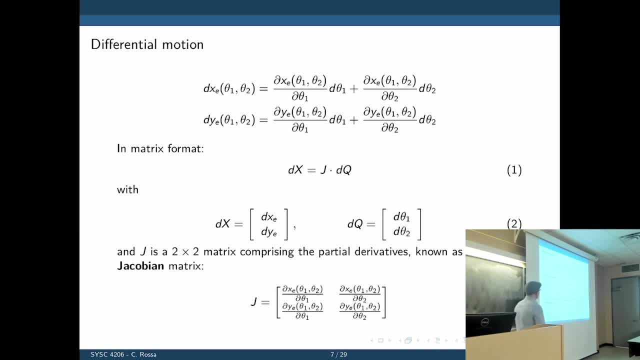 completely it. and now we can write this in a matrix format. What are the inputs to our system Are the variations of theta1 and theta2 and the outputs are the resulting variation in the tip position in the X and Y direction. So if I write: 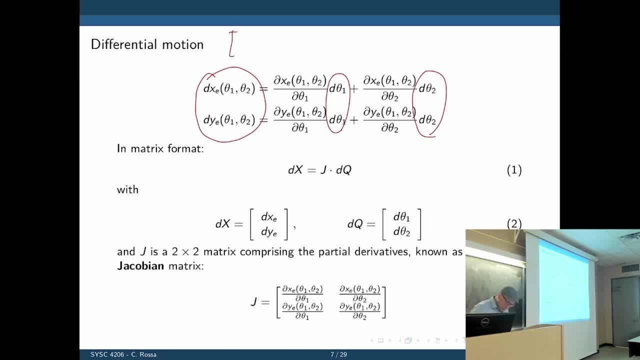 this in a matrix form. I can simply have dx Gy like that. This has a matrix in it. and then on the other side, here we have d theta1, d theta2.. Or in other words, if you call that a big space, and let's homemade that義 θ senza'. 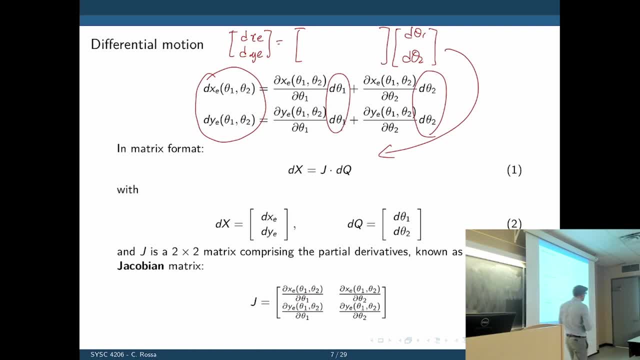 vector here dx, and then the d, theta one, theta two, just dq. Q means the variable you're controlling. What is j? Well, j is what goes in the red part there, which are these partial derivatives. So basically, take these four partial derivatives, move them there, so j would look. 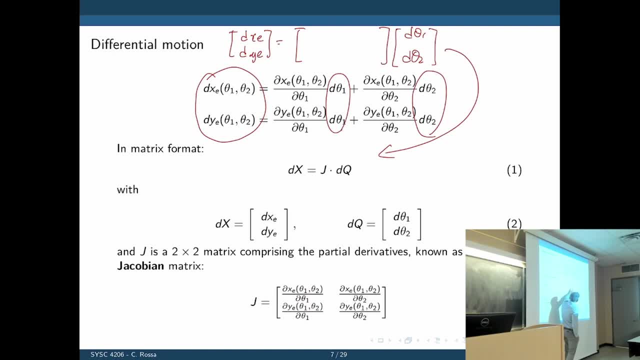 like this: Now, when you multiply j by d theta one, d theta two, we get expressions for dxe, dye. Does that make sense? Yeah, So what is j? J is what we're going to call the Jacobian matrix. that relates displacements, changes in displacement of joints to changes in displacement. 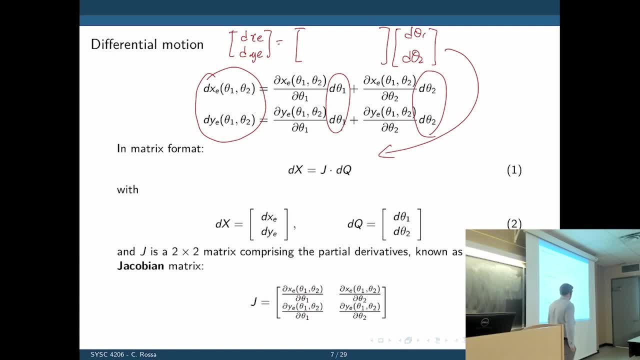 in the Cartesian position, in this case of the cartesian position. Okay, So we're going to use this throughout the class. So look at the form of the Jacobian. here We have two degrees of freedom, So you take the first degree of freedom here and 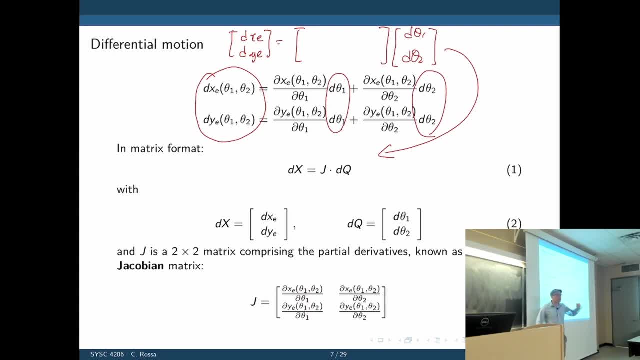 you take the partial derivative with respect to all joints that you can control, Same with the second one, and so on. Should they have a third degree of freedom? let's say the robot could also move in the y, in the z direction, then we would have a third line of freedom. 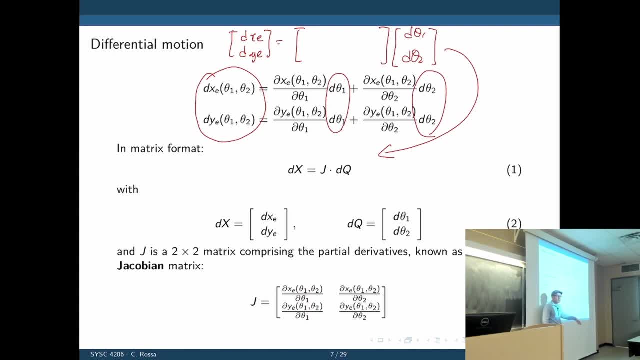 and it would be the partial derivatives of z and you would have a third actuator, so it would have another column here and it would now have the derivative of all the degrees of freedom with respect to that new actuation variable, and so on. So we will have n times. 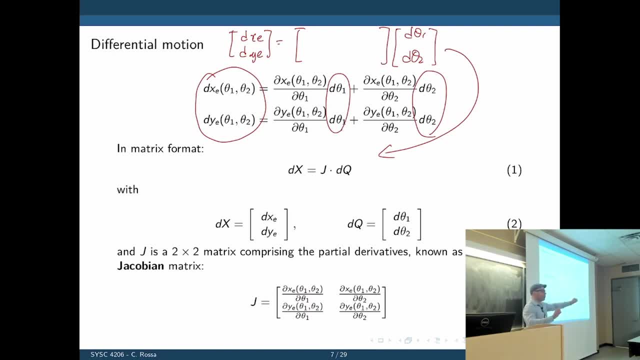 m, where n is the number of degrees of freedom the robot can move and m is the number of actuation points that you have in the robot. In this case, here is a two by two and you have a two because you have two degrees of freedom and two things that you can control. 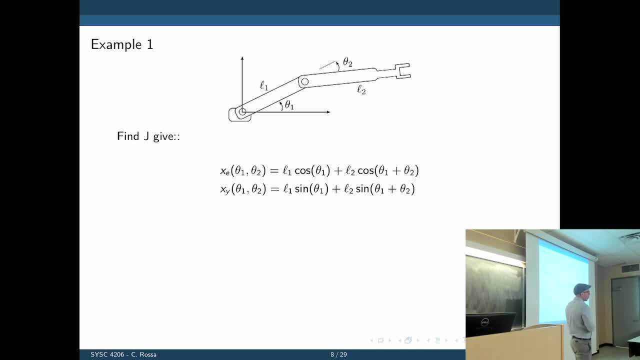 Let's do this guy here, So let's find the Jacobian for this guy now, relating the speed or the small displacement in terms of angular position to the displacement that that creates In terms of Cartesian position If we make that a delta theta small enough over time. 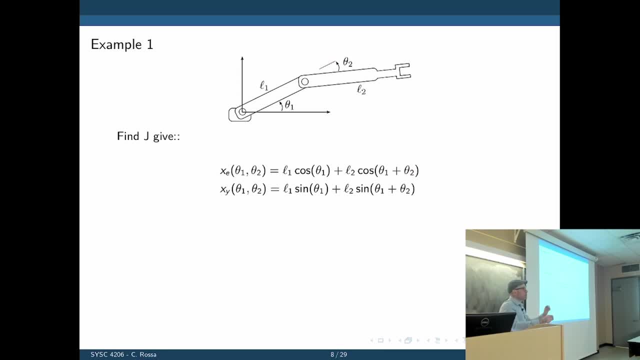 then you're talking about the derivative of position and therefore the speed in angular to the speed in Cartesian position. So what is the Jacobian here? We have two degrees of freedom, x and y, and you have three, two variables, theta one and theta two. So the 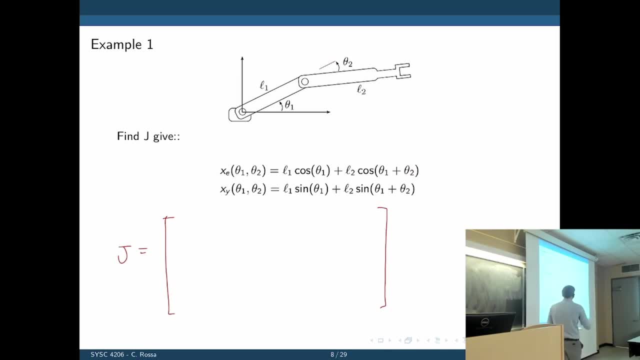 first line of the Jacobian is the partial derivatives of z. So we have n times m and we have e intended here. The derivative of z is the partial derivative of theta two, but we also need the partial of E. plus, weakness equals n times or. it's very easy to do that. 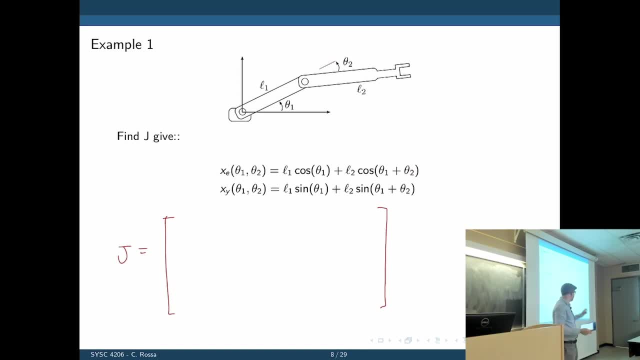 And here we had to put those two 확진 intes in here. So we've now got the partial这是 of z and then the partial throughout them with respect to theta two. together They are threemam period無. So again we need the partial derivative of Z. so we had two peruse. 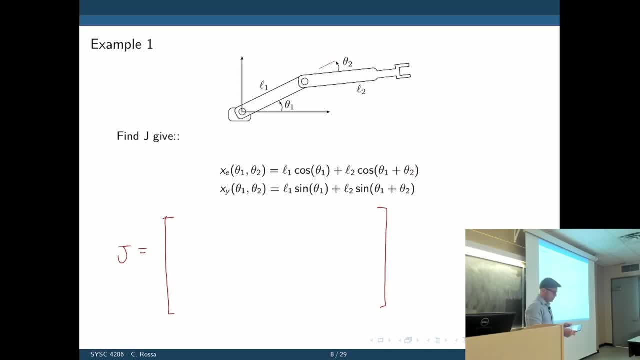 of veta. two times omega x Cosine becomes minus sine, minus L1 sine of one. It's the seg one there, Minus L2 sin Of theta. one and two, yeah, and then the second cell is the same, but now taken with respect to. 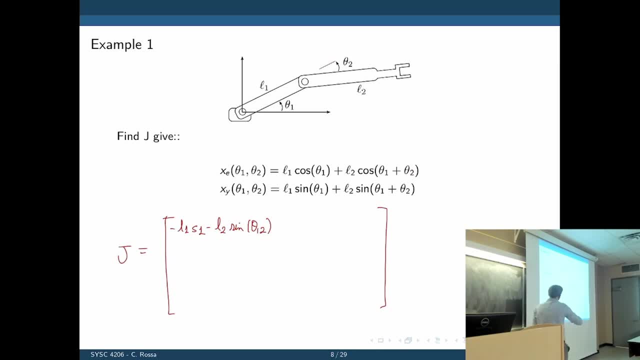 theta 2? what's the partial derivative of this with respect to theta 2: 0? and the other one is minus l2 sine of theta 1: 2. yeah, so this is partial derivative of x with respect to theta 1 and this is the partial derivative of x with respect to theta 2. 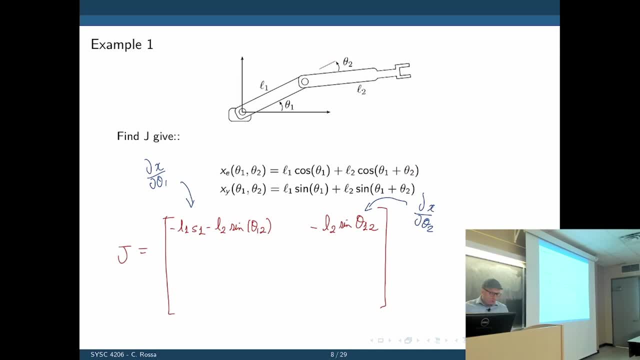 very good. are we assuming that the theta values are constant? no, those are variables. but we would do here partial derivative. so the part, the derivative of this, let's say with respect to theta 1, is the derivative of cosine negative sine times, the derivative of theta 1 plus theta 2 with respect to: 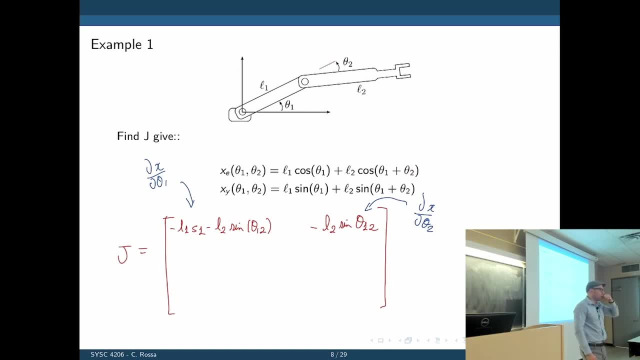 theta 1, which is 1. nice, we're always continuing the chain, but in this case it's just just 1. what's the second line? second line is the partial derivatives of y first one with respect to theta 1. what do we get? l1 cosine of theta 1 plus l2 cosine of theta 1 plus theta 2, and the other one is the partial. 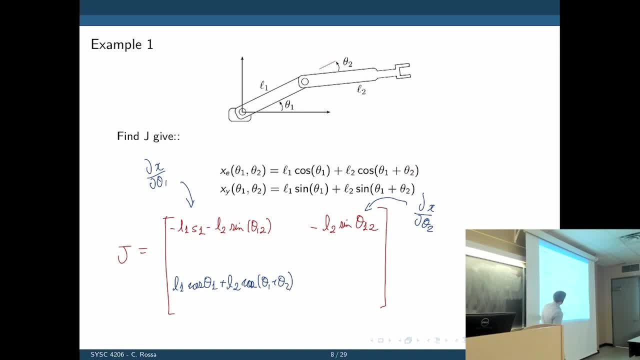 derivative of y with respect to theta 2, which is: this is 0, and that one becomes l2, l2, cosine of theta 1 plus 0, theta 2, 1 plus theta 2. okay, so that's now the jacobian relating speed and speed. now notice something important here. 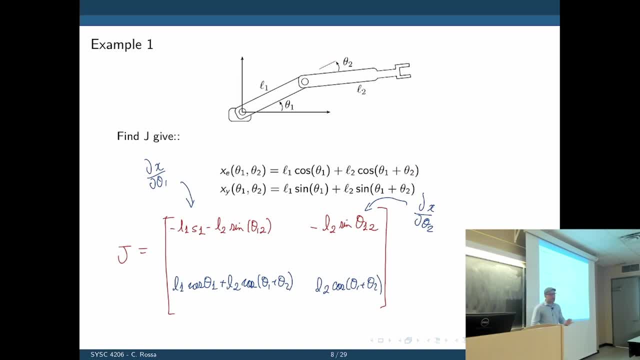 the points and the cells in this jacobian are functions of 0 and theta- 2 theta. that means that depending on where the robot is positioned, the effect of changing this applying speed to a given joint will create a different speed at the end factor and that will strongly depend on how the robot is. 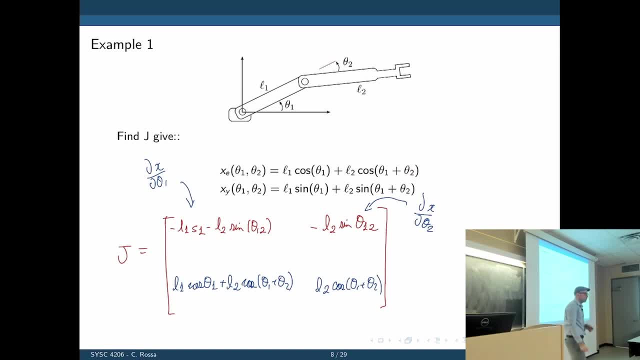 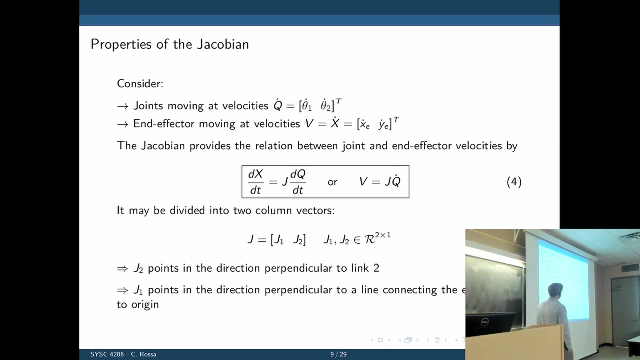 oriented. so the relation in the speed between the end factor and the joints, that strongly depends on the robot's pose. right, how it is oriented, Any questions here? No, All right, so if the joints are moving at velocity q dot, q dot is the vector with all actuation variables. In this case it's composed by theta. 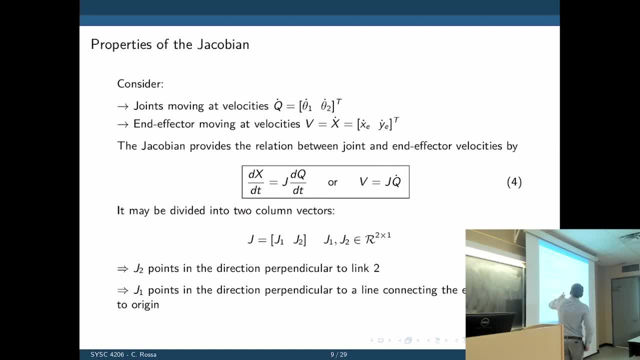 1 dot and theta 2 dot transposed and the vector is moving at velocity v, which is x dot, x e dot and y e dot. all right, It's also a vector. all right, It's a 2D space, so we want. 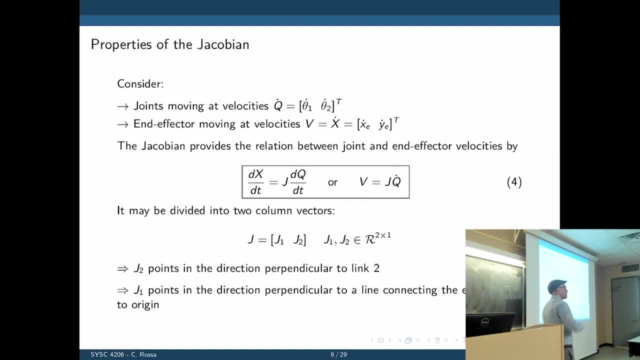 to specify the speed, the velocity. we need to specify the vector. So in this case it has a two-dimensional, it's a two-dimensional vector. So here we have, then the relation we are looking for. The derivative of x with respect to time is the Jacobian times, the speed. 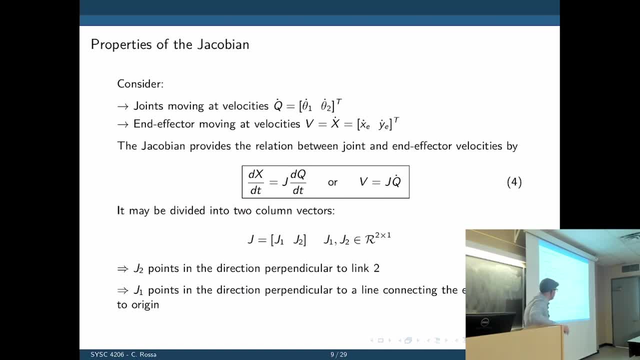 x. The speed of the end factor is the Jacobian times, the speed of each joint. The output, here, v, is a two-dimensional vector and here is the input is also a two-dimensional vector. If this was a 3DOF robot, then the speed would be expressed in Cartesian coordinates with three. 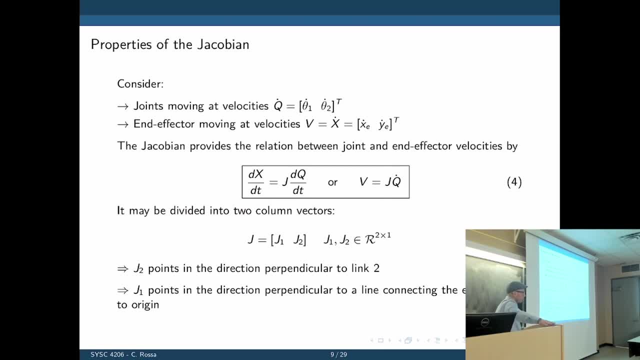 degrees of freedom instead of two. Good, Okay, so we can take this Jacobian matrix and split that into two with J1 and J2.. J1 is a two-by-one vector. so is J2.. We are forming that with two vectors. What information does that provide to us? 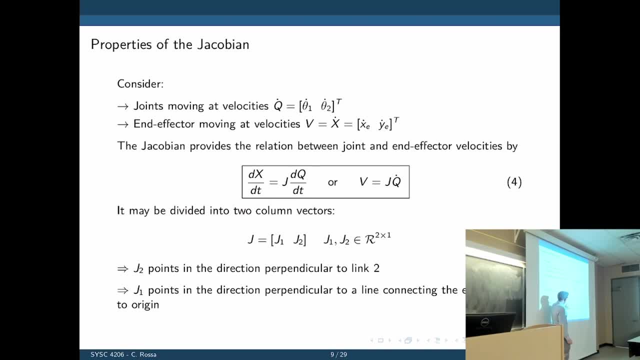 Well, if you look at, let's say, the vector form by J2, it will give us a direction. the system would move if we actually only act about theta two. So if you- only you- hold theta one static and apply a speed to theta two. 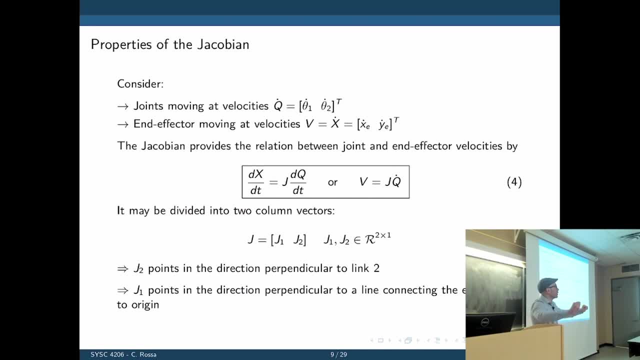 dot, theta two or theta two dot is not zero, then the robot will move in Cartesian space with a vector that is given by J2.. Same works the other way around. If we make theta 2 static and you apply a speed to theta 1 dot, then J1 gives the direction in which the robot moves in that particular case. 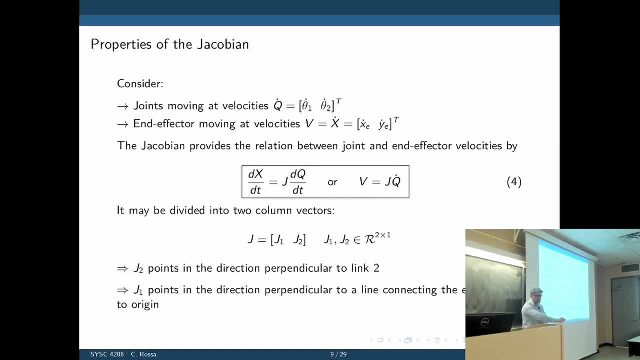 all right. So in other words, let's assume that we have this 2-dof arm like that And J2 gives points in the direction perpendicular to link 2.. So if I only actuate my elbow, you see that the speed here is always perpendicular to my hand right. So the vector in J2 is always 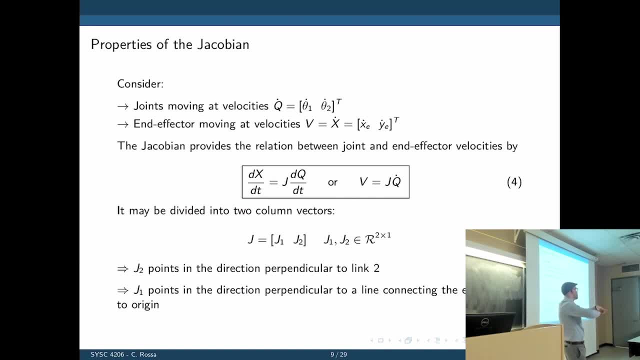 perpendicular to the second link. in this particular case, How do we find J1?? Now J1,. I'm holding my elbow static and I'm applying a speed here, all right to the other joint. What should J1 be? J2 is 0, right, Theta 2 is 0.. No, the elbow is not rotating this way. 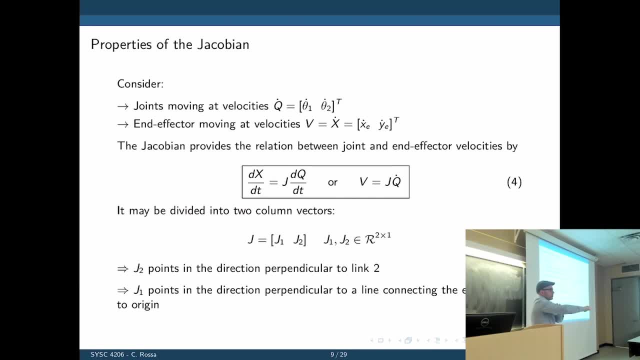 But you're moving the J1, so that means you're moving the elbow as well. right, So you're moving the end of vector. These are- we are looking at positions of the tool tip, only speeds of the tool tip, all right, So if I move it like that, it doesn't matter. 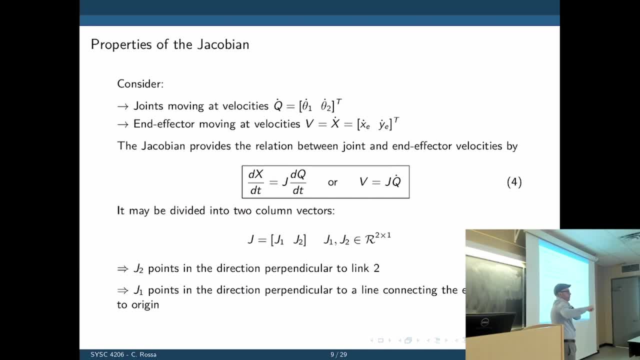 This is fixed. I'm just applying a rotation here, all right. So in which direction does it move? It moves in a direction that is perpendicular to a line that goes from my shoulder to my hand, right On an angle like that. Let's see an example here. 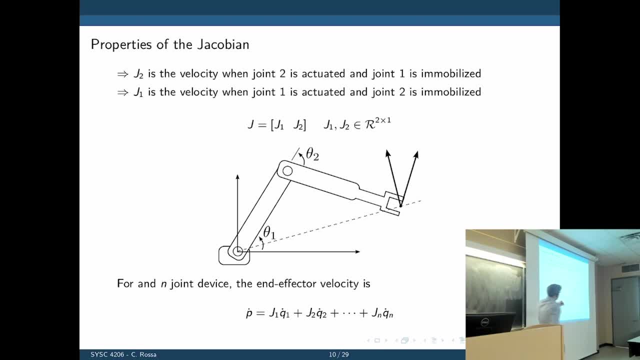 Let's do the robot first. So J2 gives the position- excuse me, gives the direction of motion or the speed when theta 1 is 0. So if I move it like that, it doesn't matter. Theta 1 is fixed and theta 2 rotates. If that is the case, then the robot should move in this. 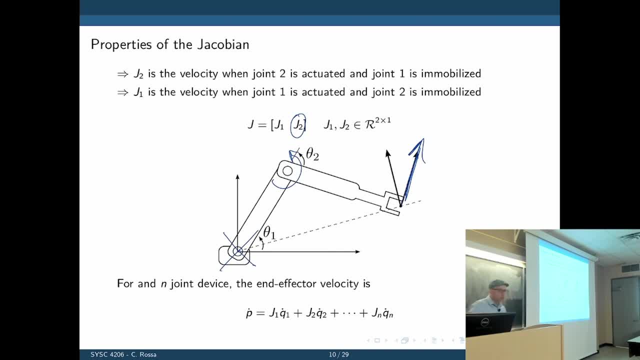 direction or back right, So that vector there has X and Y coordinates and is given by J2.. In the same way, if I now fix theta 2 and apply speed to theta 1 here, all right, The robot now becomes this line: 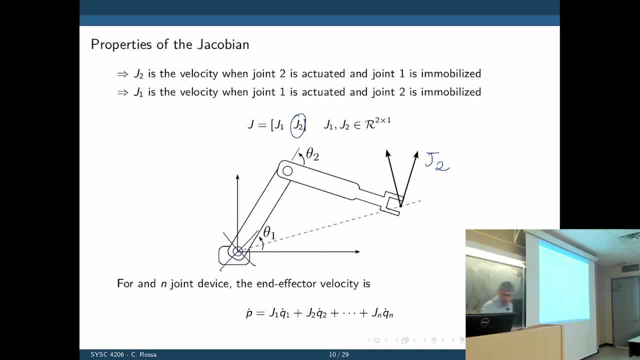 Because this can move. So now the speed of the robot is given by J1. that is found by tracing a line from the base of the robot to the tip, and then J1 is perpendicular to that. Does that make sense? Yeah, So what happens when theta 1 and theta 2 are both non-zero? 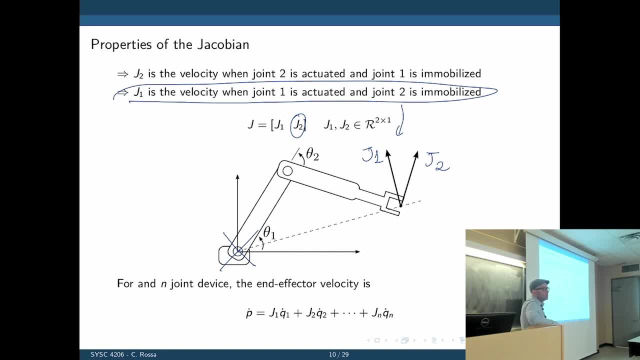 What's the final speed? Is it a linear combination of the two vectors that we scale up and are down? all right, By changing now the individual actuation, the speed of individual joints. So you see here, the total speed of the end factor is J1, Q1 dot, J2, Q2, dot, J3,. and so on. So you see here, the total speed of the end factor is J1, Q1, dot, J2, Q2, dot, J3, and so on. So you see here, the total speed of the end factor is J1, Q1, dot, J3, and so on. 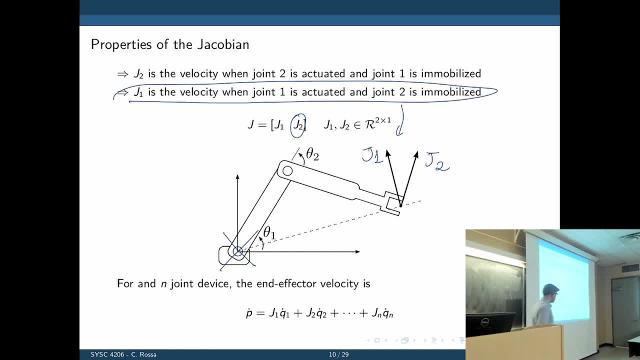 All right, It's a linear combination of all of them. Does that make sense? Sure, 100%. This is a very important topic. We'll come back. It's always going to haunt you until the end of this class now. So if theta 1 and theta 2 are rotating in the opposite directions, there won't be an effective structure. 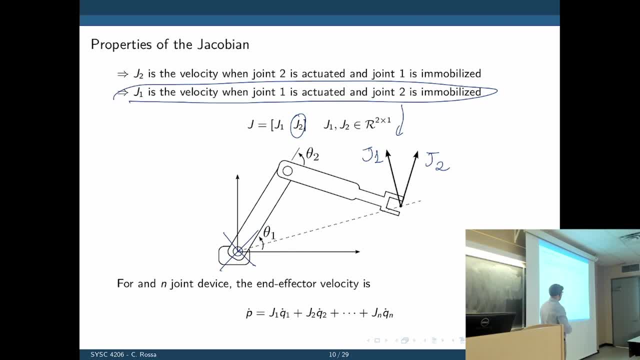 There is always. There is always going to be an effective vector, but we are scaling, So let's say this is going to be it right. Theta J1 and J2 are fixed based on the robot's orientation. all right, So these two are constant. 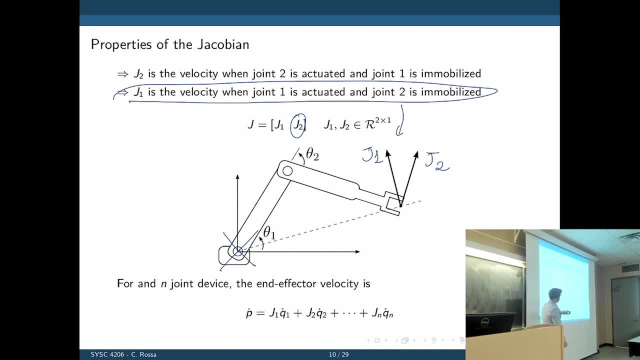 Now Q1 dot or Q2 dot can either be positive or negative, but we're still adding them up. We don't know what is in J. It could very well be negative as well. So there is going to be a resultant speed in a given direction. 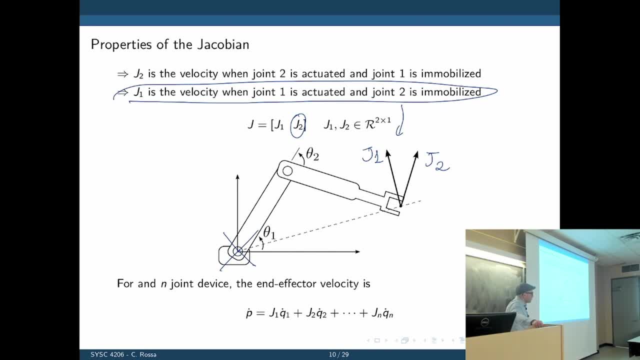 Okay, Yeah, So that one is for a linear combination. Yes, Okay, Yeah, So that means it is actually adding all the vector here. Sorry, say that again. It's adding all the J's together, scaled by the speed of individual joints. 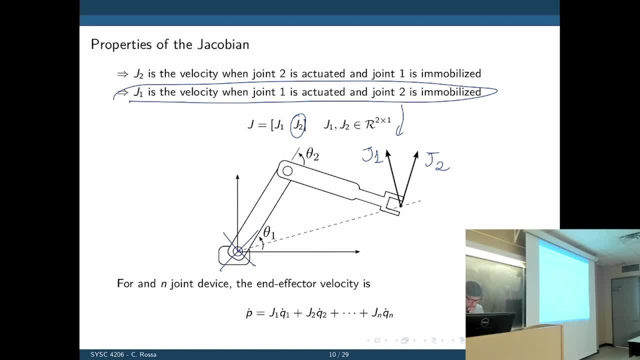 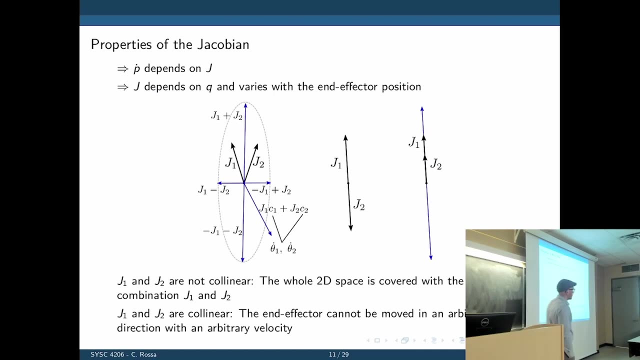 Scaled by the speed of individual joints. All right, So let's make things a bit more interesting, Sorry. Let's see what the Jacobian actually tells us. We know fundamentally. what it's telling us is the relation between the speed angular and Cartesian speed. 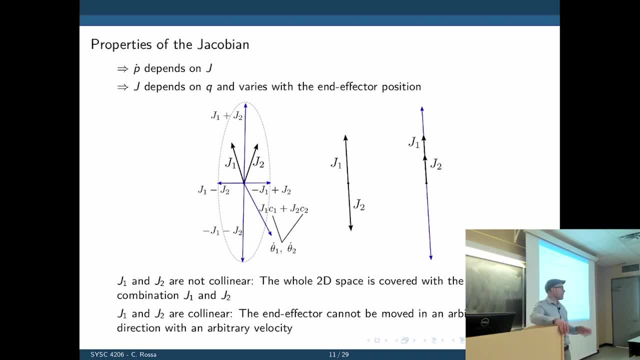 We know that now each column in the Jacobian provides the explicit relation between a specific joint's speed And its influence on the Cartesian speed of the end effector. So for our 2D two-dimensional robot there, these are all possible combinations that we can achieve by combining J1 and J2.. 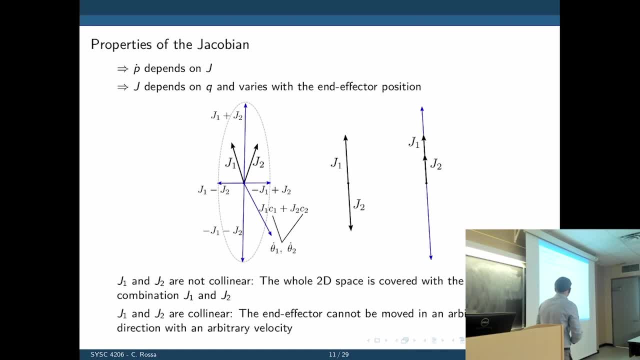 By combining the roles of the Jacobian When they add up perfectly like here. So theta 1 and theta 2 are 1.. We can have them adding up, We can have them added. like that. We can have one opposing the other, as Miles suggested. 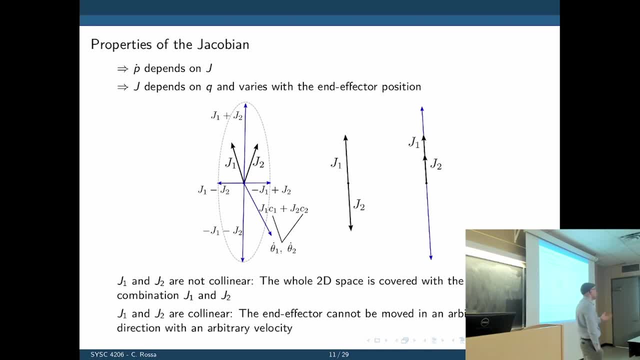 But it's still not necessarily 0. Because J1 and J2 may not necessarily be the exact same size. And then here we have their possible linear combination. So anything within that ellipsoid, any direction, can be achieved by combining theta 1 dot and theta 2 dot. 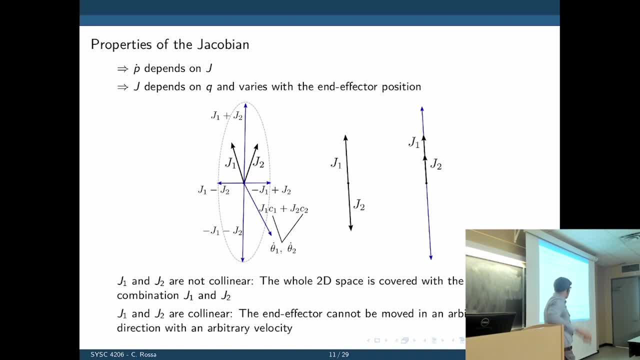 So so long as theta 1, excuse me, J1- and J2 are not collinear, Let me repeat that So long as J1 and J2 are not collinear, the robot can be moved in any arbitrary direction, Because it can simply scale them up or down. 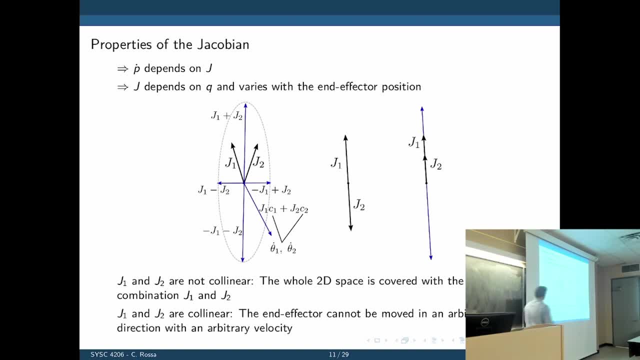 So that's what you see here. Let's say J1 is that J2 is pointing up. I can achieve any combination of them by now scaling individual J1 or Js by multiplying them by the speeds that you have control of. So that only works if they are not collinear. 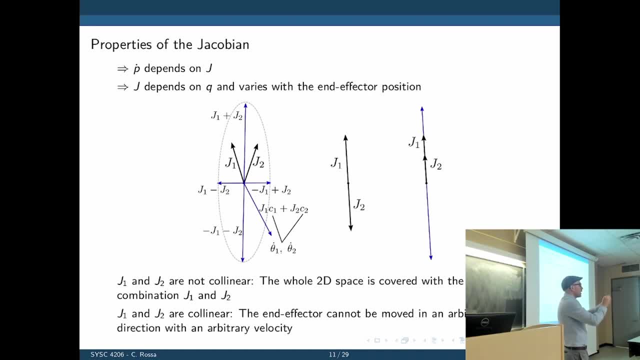 What happens if they are collinear? Well, if they are collinear, I can stretch them one way or the other way, But I cannot change their direction. Regardless of how much I scale them up or down, the result is always along the same line. 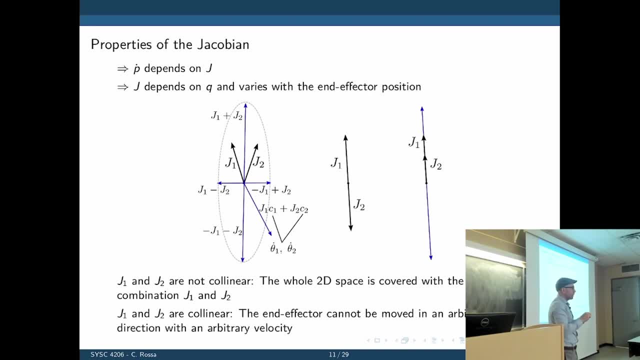 Does that make sense? Yeah, Alright. so let's do an example on the board here. Let's say we have J1 like that and J2 like that. Alright, what's the sum? It's this. This is the final speed. 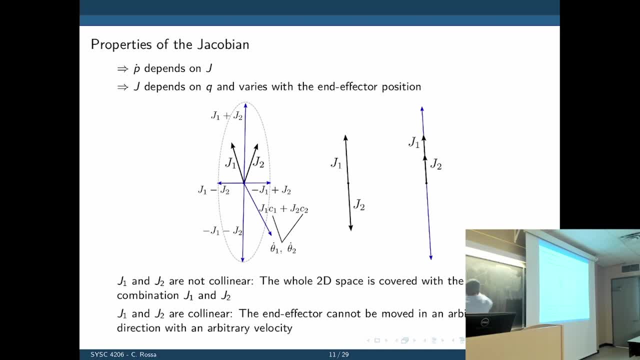 But I can multiply. Remember that these have to be multiplied by theta 1 dot and theta 2 dot. So I can scale this guy here As much as I want By simply multiplying that by theta 1 dot, By controlling the speeds of that, or even the same in the other direction. 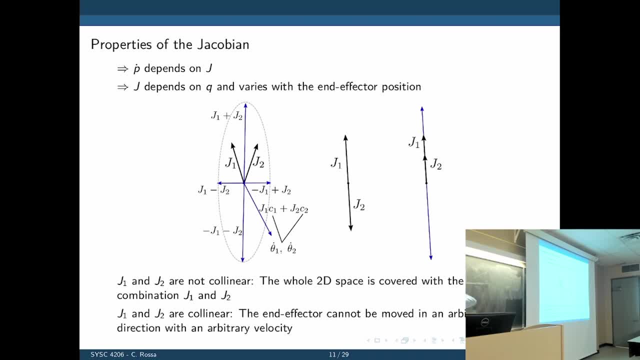 Alright, Which means that if I keep this one static, my speed now can be anywhere here. Does that make more sense? Yeah, Alright, so let's say this is the original vector. My speed was here. Now I double the size of this one by simply doubling the size, the amount of speed I applied to theta 1.. 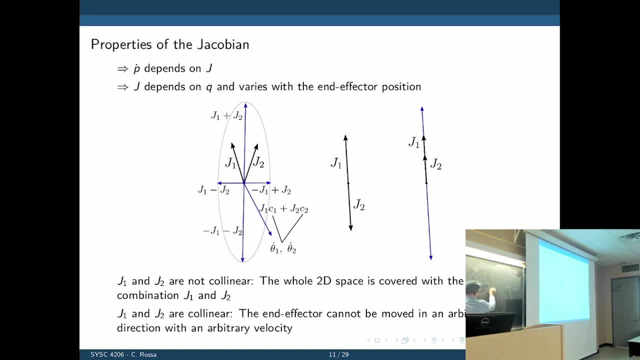 What's the final speed now, Or the end of the vector? It's like that. Alright, If I wanted to move even more in that direction, I can reduce this speed, In which case it will move like this: Yeah, Every direction. 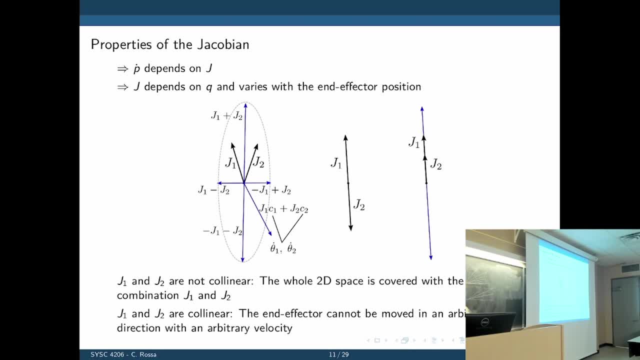 Because I can also flip the direction off of them Alright, By reversing the speed. So this works fine, so long as they are not collinear. What happens if they are collinear? Now I have theta 1, let's say J1, pointing that way. 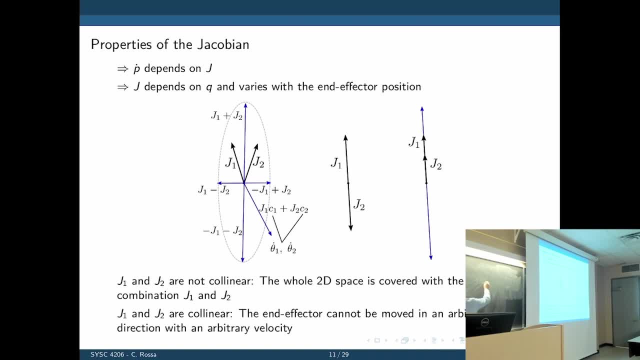 If I scale J1, in which way can I scale it? That way or this way, Alright Along that line? If I have J2 pointing this way, This way is the same. So the resulting vector, regardless of the size of J1 or J2, will belong to this common line between them. 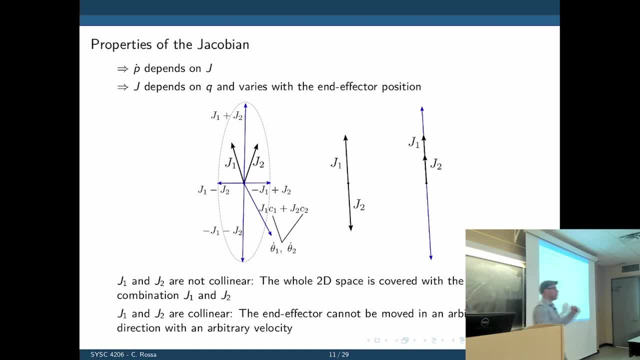 Alright. So if they are collinear, they can only move in one particular direction. What's the problem with that? Well, the problem is that you lose control of the robot in other directions. We can only move along a certain line. 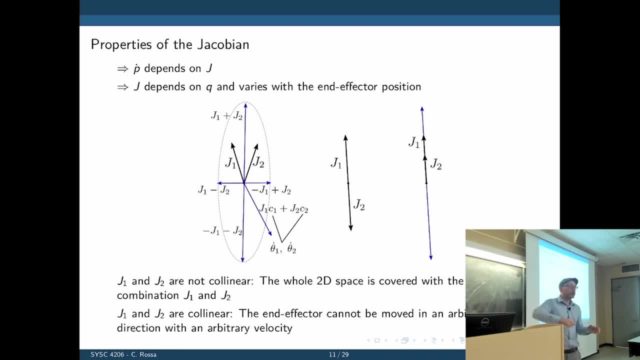 And that's what we call a singular configuration. That's the singularity of the robot, And the Macademic has a bunch of them. You've probably noticed a mysterious error at some point. Well, it just means that you've probably done it. 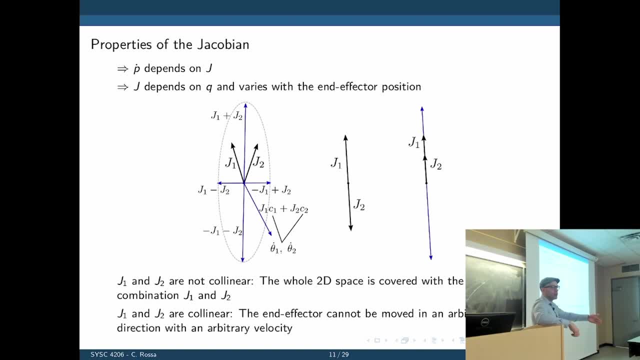 You've probably put the robot by accident in a singular configuration and asked it to move in a direction that it can't Alright Because of what we see here. Now, in the case of the Macademic, it's a much more complicated problem because you have six of these individual J's. 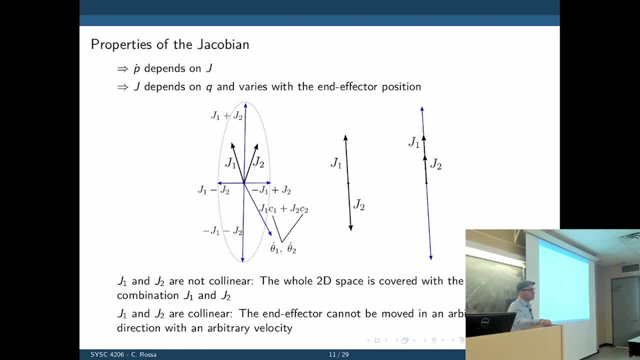 And the Jacobian is a six by six matrix, Alright, So it's a little harder to see where these singularities are When the J's are aligned. No, not all six, At least two of them, Yeah Yeah. 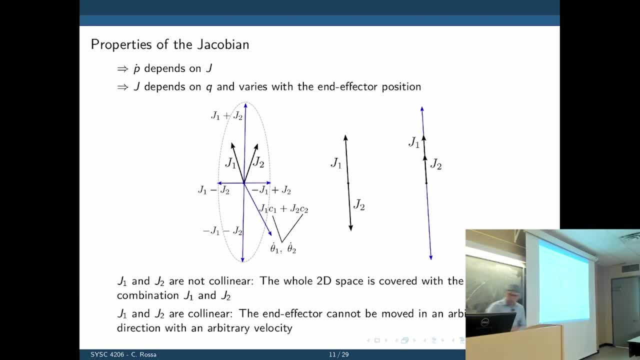 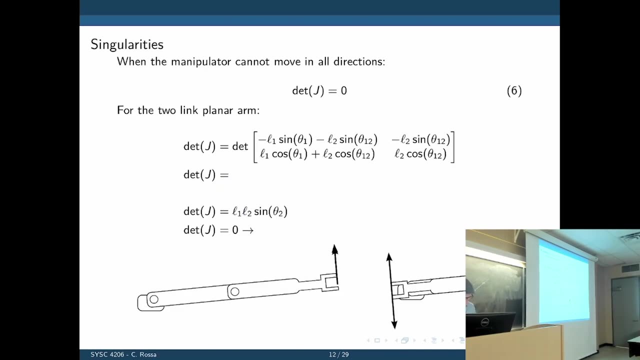 Alright, Alright, So that's what a singularity means. So you're losing the ability to move, To move in a specific direction in Cartesian space. Okay, So let's look at our example. Back to our example here. 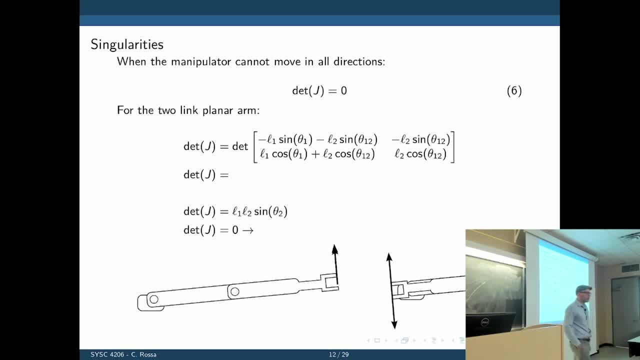 What is the determinant? Sorry, Let me. Why am I talking about the determinant? To find the singularity. it happens that the singularity will occur when the determinant of the Jacobian is zero. Easy Right. When the determinant of the Jacobian is zero, the robot is in a singular configuration. 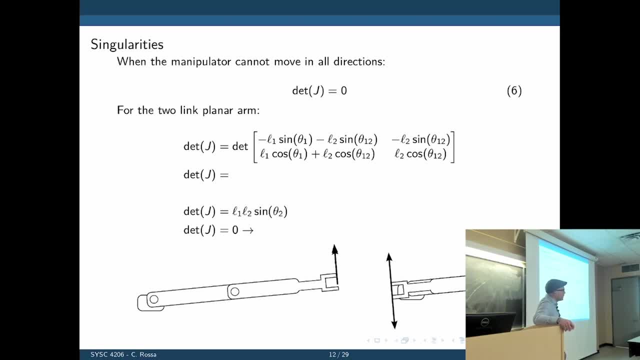 So for our Jacobian that we just calculated, what is the determinant? Is this times that Minus Minus, This times that That times that Right. So what is? it Is L1. Minus, Minus. 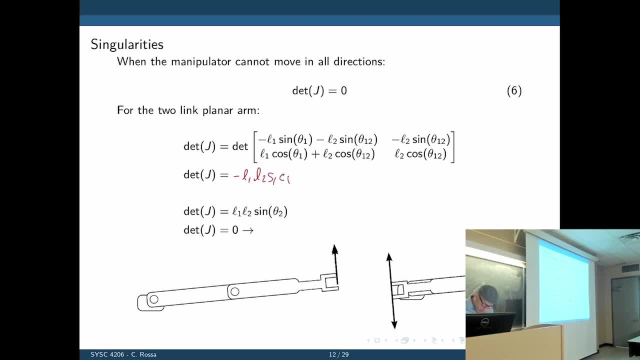 L1.. L2. Sine 1. Cosine 1. 2. Minus L2.. Squared Sine of 1.. 2. Cosine of 1.. 2. Plus L1.. 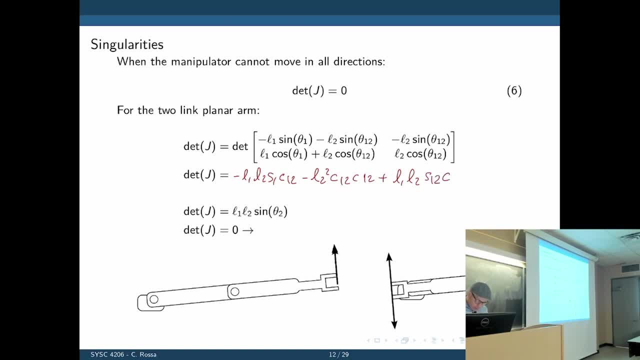 L2. Sine 1.- 2. Cosine 1. Plus L2. Squared Sine 1.- 2. Cosine 1.- 2.- 2. L2. Sine of 1.. 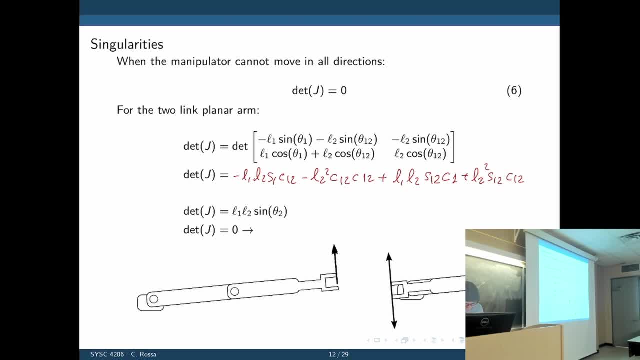 2. Los 1. L2. L1. Ni 2. Minus Minus L2. L3.. So we got equal 5. We got 1.. Okay, So I'm now going to go through the details, but that's the determinant. 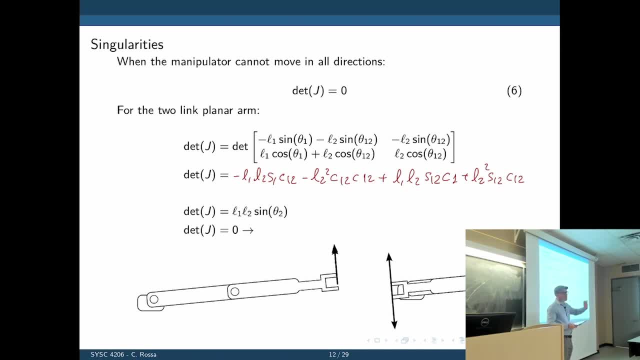 And now, if you use some trigonometric analysis- I'm going to skip that part- We can simplify this whole expression using some magic during the midterm. to that configuration there, to that expression: L1, L2, sine of theta 2. How do we make that zero? How do we make that zero Theta? 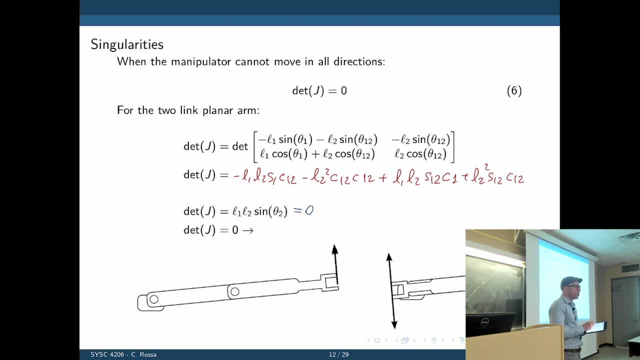 of 2 must be either 0 or 180.. So if theta 2 is 0 or 180, the robot reaches a singularity, because the determinant of this Jacobian is 0. Does that make sense? Well, let's look at the orientations of the robot. where? 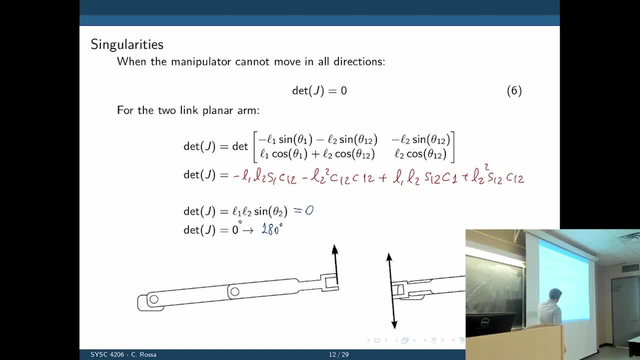 theta 2 is 0, which is in this case. here the robot is simply fully stretched. Both arms are fully aligned. If both arms are fully aligned, J1 and J2 point in the same direction. All right, so you can make an analogy again with my arm, If I have my arm. 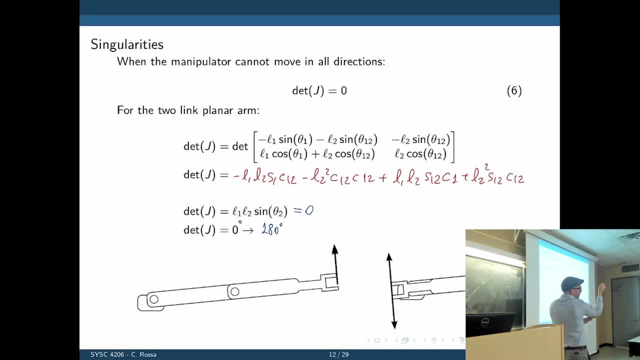 fully stretched and I move and I rotate my arm around my elbow or around my shoulder, the resulting speed is in the exact same direction. So this is a singular configuration, because that's basically the only direction we can move along. The other configuration is 180.. So this: 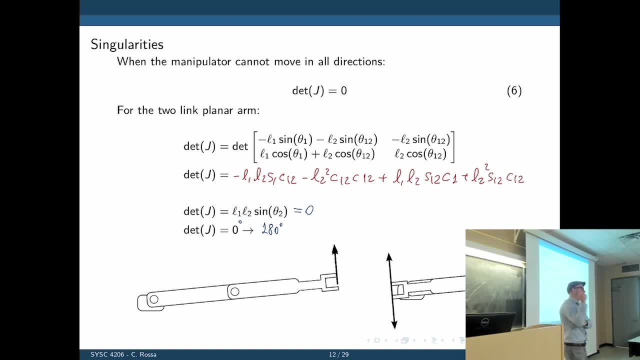 our arm is folded on itself, and it's the same problem, except that now J1 and J2 are opposite, All right, and if they are opposite again, doesn't matter how much we scale them up or down, we are scaling them along the same value, which means 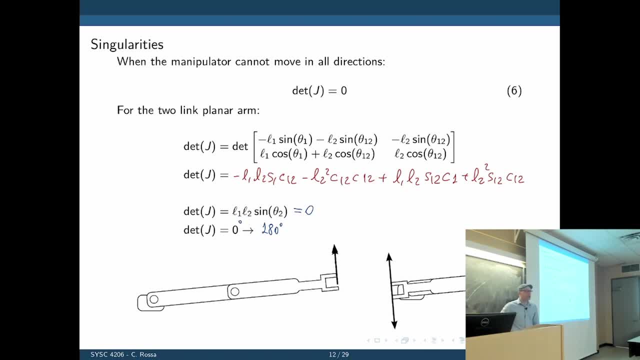 that now we can only move along that line. So the only purpose of the determinant is to basically verify the singularity of the robot. Yes, and you want to keep the robot away from this singularity, Excuse me. so in the third step, is that L1, L2, sin-theta 2 equal 0?? 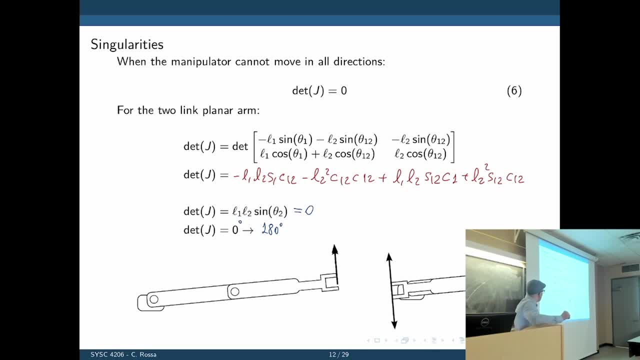 Yes, And how about the last step? What is the, the l- singer in the data items are negotiating? That means yes, that means that the determinant is 0, if sorry, it means that the determinant is 0 if Theta 2 is 0 or Theta 2 is 180, yeah. 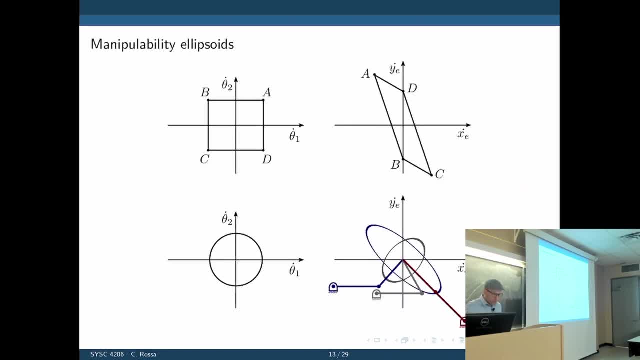 Okay, Good, All right. So we know what this Jacobian is doing now. it's doing a mapping between the speed in the joint space- not in the joints- to the speed of the Cartesian space, the tip of the robot. 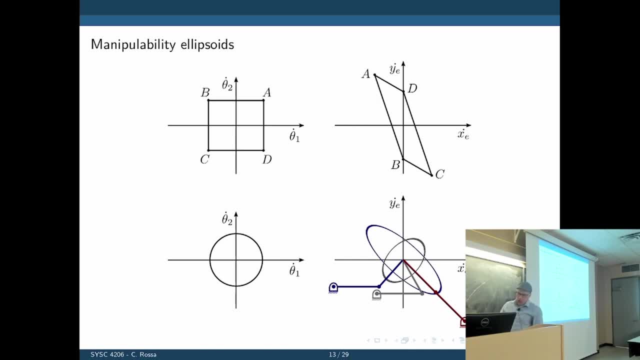 So we could see how that mapping changes the speed or creates a speed in the robot by inputting or passing through the joints Jacobian all possible combinations of speed that the robot can take. So if you plot here Theta 1 and Theta 2, and these points here are the maximum speeds. 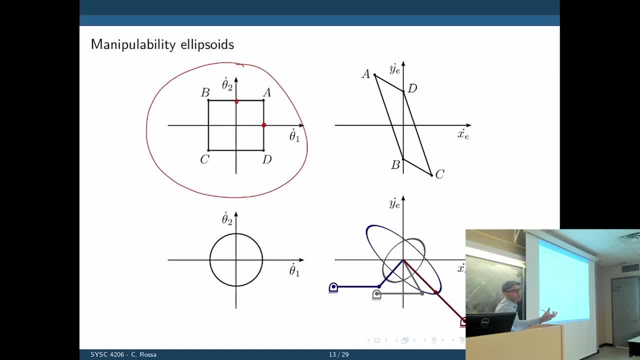 of each individual joint, this maximum feasible speed of each individual joint. We can take any combination within this square. Any combination means a specific value of Theta 1 and Theta 2.. We give that to, we pass that through the Jacobian and we see the resulting speed of. 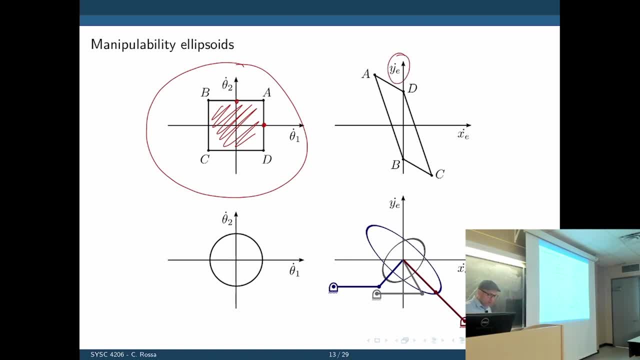 the endorphin And you see that the resulting speed of the endofactor is also in 2D. it's X and Y dot, like that, And you can then plot the resulting speed in Cartesian space. So let's say we take point A. point A gives the speed of Theta 1 and Theta 2.. 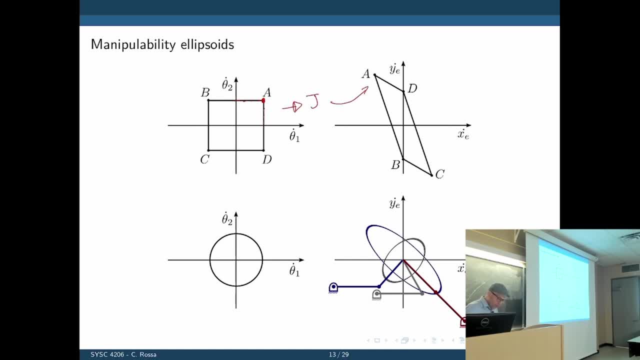 We pass that through the Jacobian of the robot and we get the equivalent Cartesian space there. This mapping only works for one specific configuration of the robot, because as soon as we change the pose of the robot, J changes and the mapping again changes. 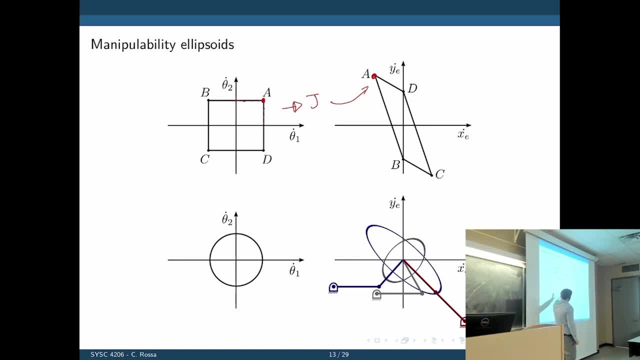 So it's more common, when you look at robotics textbooks, to, instead of defining the inputs in a square like that, we normalize Theta 1 and Theta 2 with a circle in a way that this is the radius of that circle is always 1.. 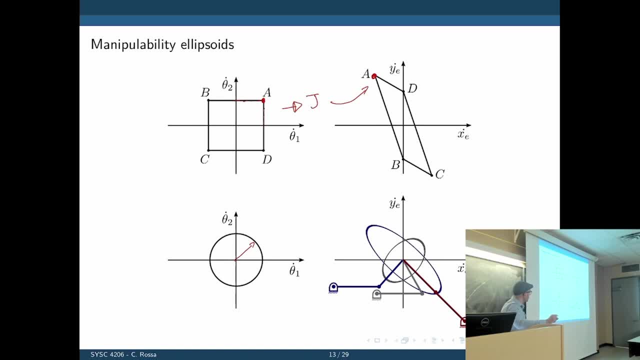 It's always 1.. And then you pass that through the Jacobian again and you see what is the feasible range of Cartesian space speed. So if you take this point, we pass that through the Jacobian and we plot that point, let's. 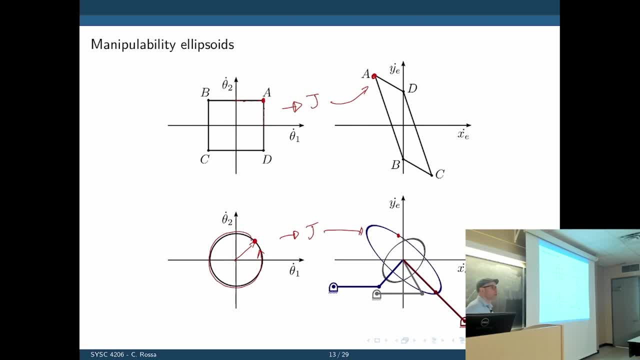 say here, Then this point now revolves around the circle and you find the equivalent point on the other side, And that will give us this, This ellipsoid. Now notice something: If the robot is in this configuration, this is the speed ellipsoid. 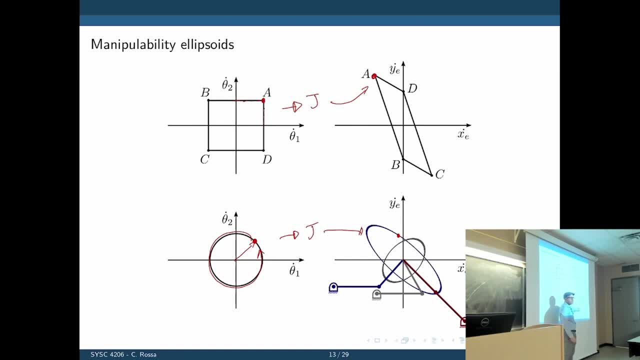 If you change the robot to that configuration, that's the speed ellipsoid. If it goes to that configuration, then it's a different ellipsoid It strongly depends on because the mapping is done by J, and remember that J is a function of Theta 1 and Theta 2.. 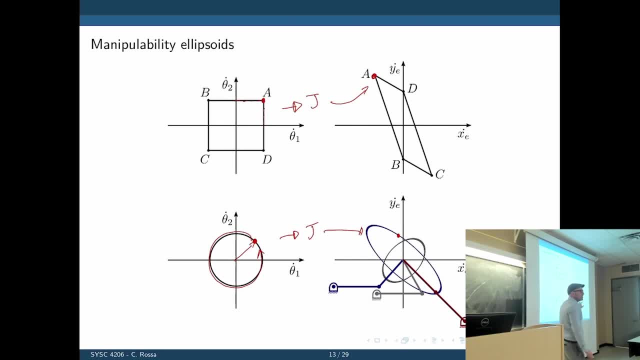 What happens with these ellipsoids? when the robot is in a singular configuration, They become a line. right, You squeeze it to a line because it can only move along a line, all right, All right, I'm sorry. can you explain something about that one? 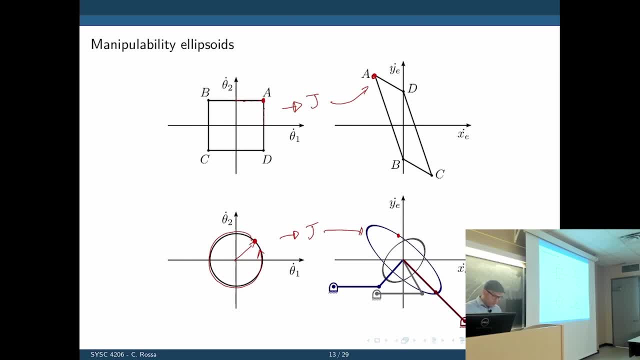 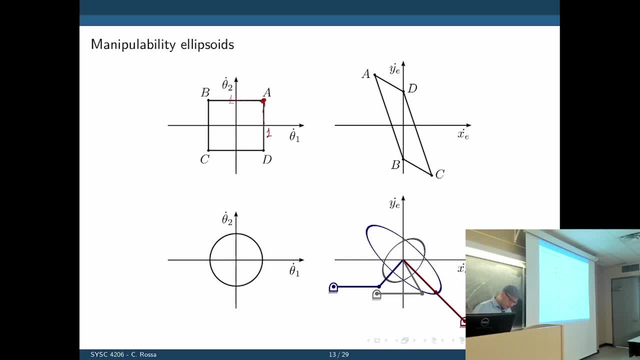 Theta 1, let's say of one radians per second speed, into two of one radians per second. We know that the Cartesian, the Cartesian speed, is J times Theta dot. So we take these two Theta dots, We put them here. J is a function of Theta 1 and Theta 2, then we get V. V is a two-dimensional. 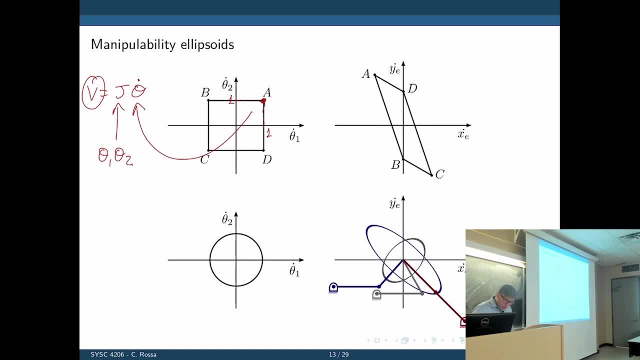 vector that has X and Y. Let's assume when you plot X and Y speed it falls there. So then that is the equivalent point that it gives the direction of the speed in Cartesian space, Because we don't know what J is right. 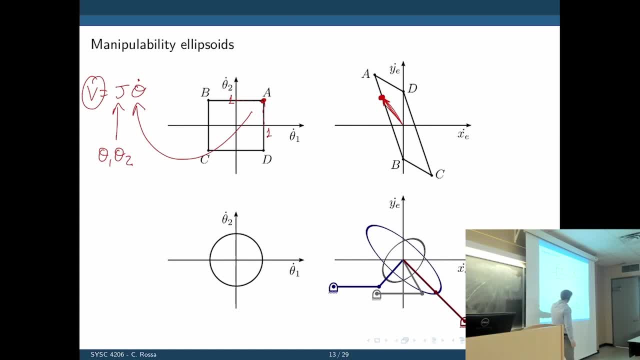 It could be anywhere. It really depends on J. In the same way that this ellipsoid here will strongly change, well that one also will change as soon as J changes right. So the manipulability of the robot strongly depends on its current pose. 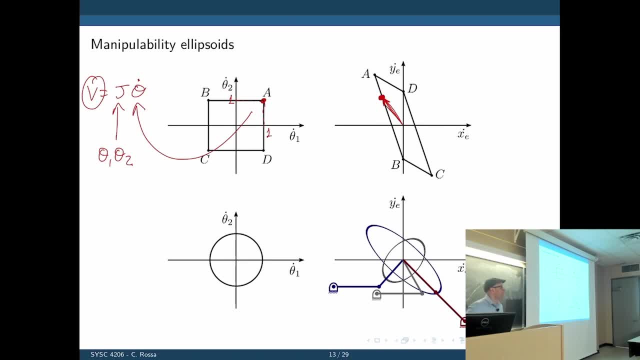 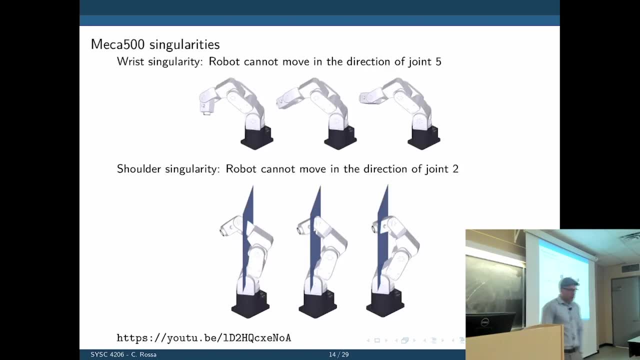 Yeah, All right. so here we have some of the singularities with the macadamic robot. I have a YouTube video here that shows all of them, but I selected only a few here for us to look. So the first one: I have the top there. those are three singular configurations where the 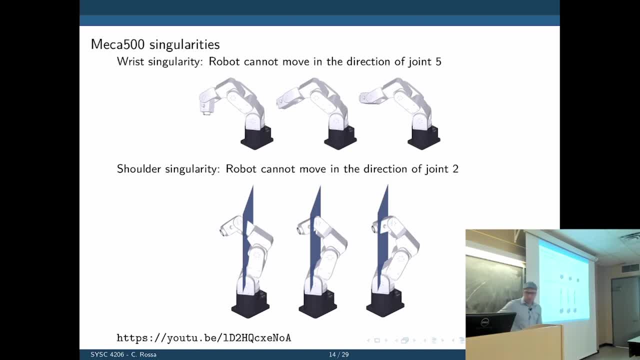 robot cannot move in the direction of joint five, here joint 1,, 2,, 3,, 5.. So in this configuration the robot cannot move. the tip of the robot cannot move along that line. If you wanted to move along that. 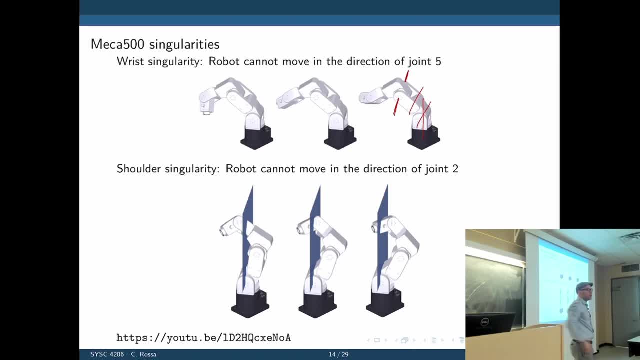 line. you first have to reorient it and then slide it along that line. So there are three possible ways to put the robot in that position. Here are- here's another one- These three configurations. in these three configurations the robot cannot move in the direction of joint 2. So anything along the plane there is not. 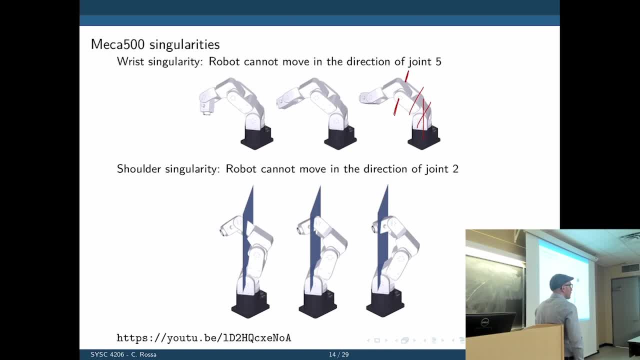 feasible. The tip of the robot cannot move, cannot create a speed in that direction. But the problem here is a lot more complicated, because you're dealing with now six degrees of freedom instead of just two that we saw before. Well, that depends on each individual joint운� features. 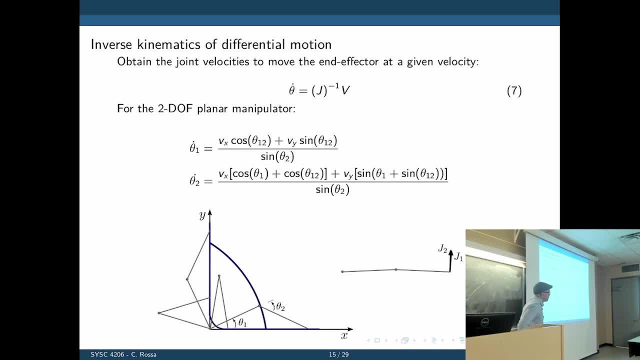 Ok, now let's do the opposite. We know that by changing the speed of individual joints we achieve a certain speed in the end effector. Let's try to do the opposite. If we want a specific speed of the end effector, what? 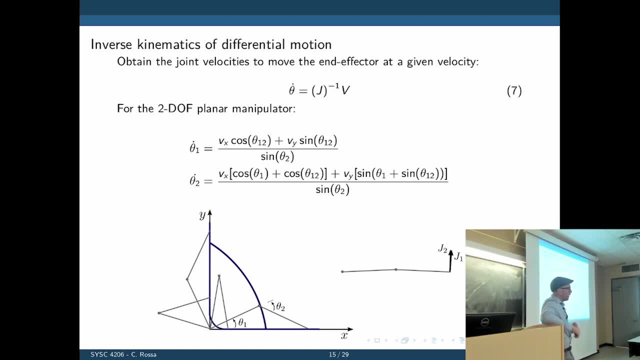 is the speed of the joints that we need to achieve that. Well, it's just the inverse of what we did. we move the Jacobian to the other side, we invert it, and now we have: we specify V, we specify the desired Cartesian speed and we get the required joint. 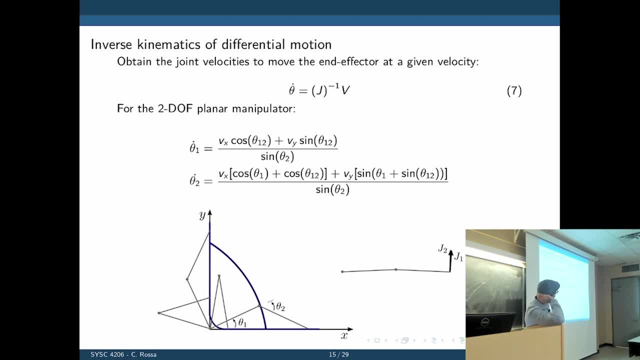 speed. So if you do it for the robot we just saw, that's the expression we get. Do you see a problem with that? We see that that is divided by sine of theta 2.. When theta 2 is 0 or 180, that 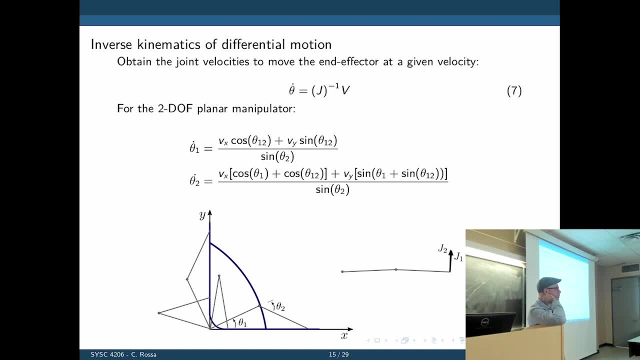 goes to 0, the whole thing blows to infinity. So when the robot approaches its singularity, the ability to generate a speed in that particular direction requires more and more speed in the corresponding Cartesian joint, to the point where it will tend to infinity, because the robot approaches a singular value and 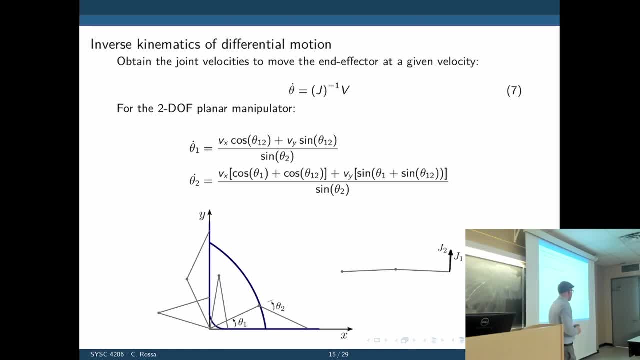 cannot move along that direction. So you see the problem happening mathematically right here and you can try to make sense of it if you give the robot this blue line to follow and you see the different orientations of the robot as it tries to follow that line at a given constant speed. let's say 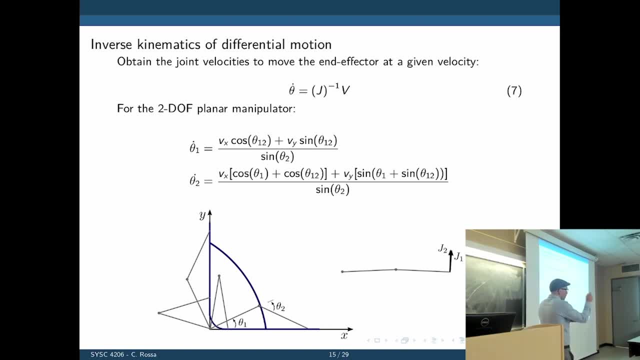 It's a constant speed. It's a constant speed, Give it a constant speed, but I want it to move along those lines at that constant speed. What is the required speed of theta 1 and theta 2 to achieve that? So, so long as you. 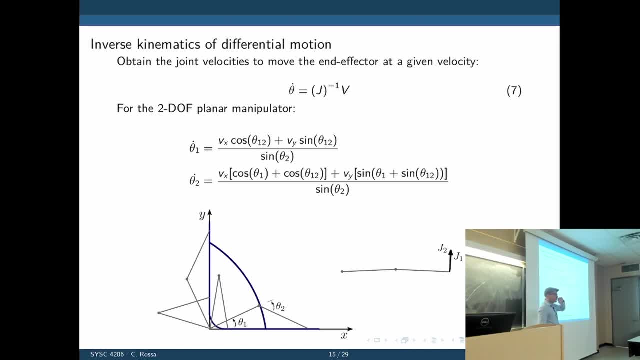 are away from a singularity. this is fine, This is perfectly feasible. But when you approach, let's say, this point over here where the arm now needs to be fully stretched, or this point here where the arm goes up and down like that and it's folded on itself and you 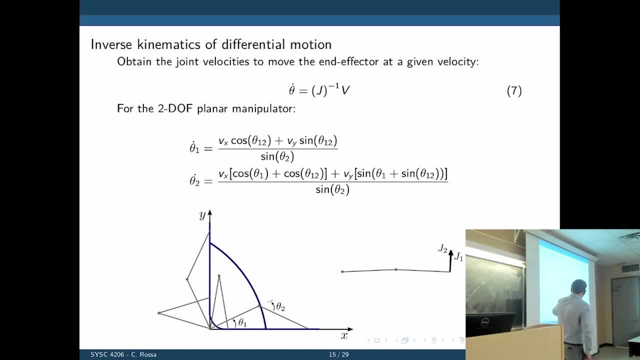 have 180 degrees for theta 2.. What happens? The speed of theta 1 and theta 2, the required speed will blow to infinity, because you're now dividing that by a very small value. But it also makes sense if you want to. 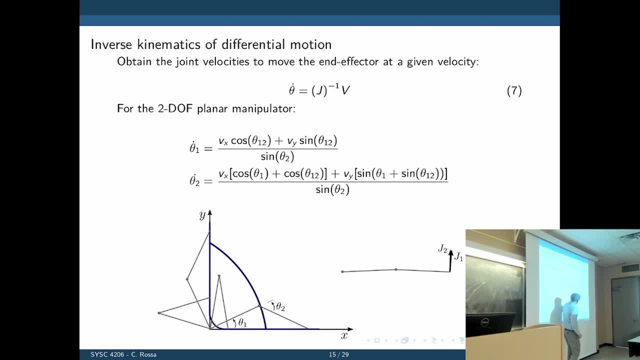 generate. let's put a. let's look at this one here. I want the robot to move that way, right, But in create a speed in that direction, because I'm moving that way, The farther I go, the closer the robot is getting to a singular value, right, And the more I go, the more straight. 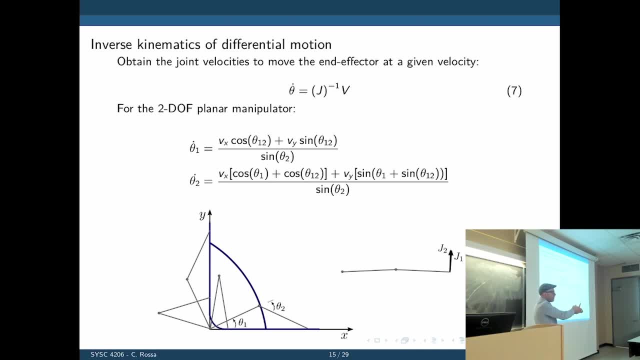 up, J2 is becoming. If I want J2 to point that way, because that's eventually the way I want to go, what I have to do I have to scale J2 and J1 in a way that the resultant force goes that way. So I'm using basically the projection of J2 and J1 on the x-axis. 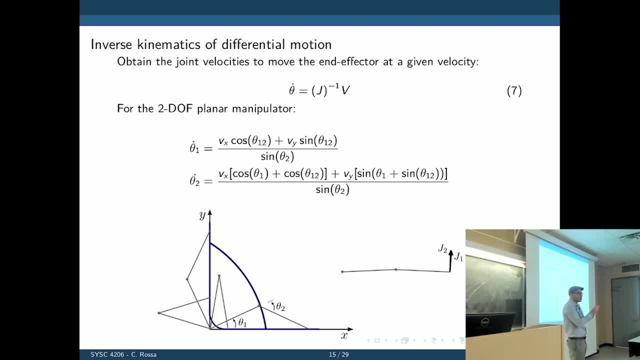 But it gets to a point. then the projection is so small that at the scaling factor required to move in that direction we'll have to blow to infinity right So that. so we can try to make physical sense of it. but you can also. 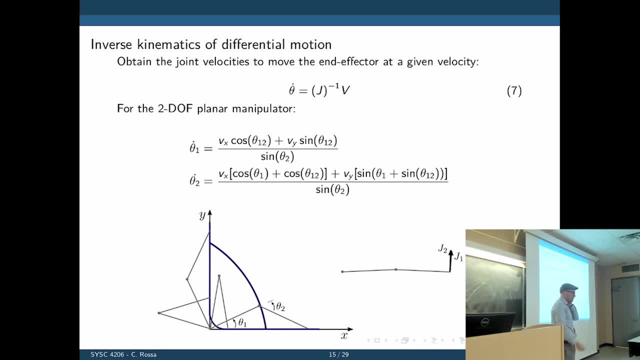 see this from the equation, because eventually, again, what you're trying to do is using the projections of J1 and J2 on the direction of motion and you're scaling J1 and J2 so that the resultant go along the direction of motion, But when J1 and J2 now tend to be, 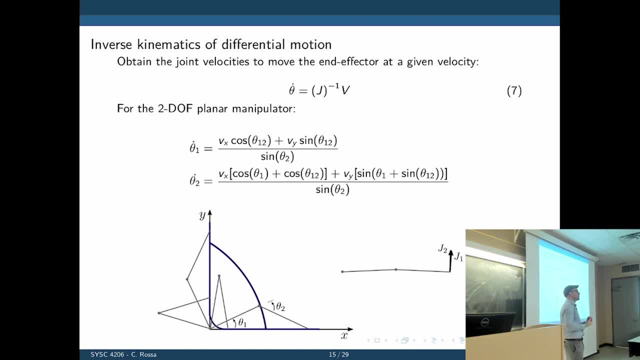 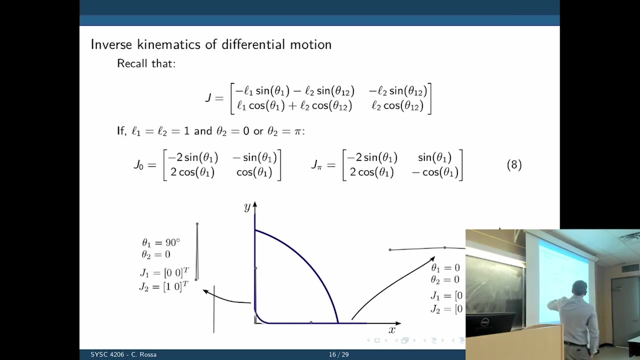 orthogonal to the direction of motion, then it would require an infinite speed to get any projection on that line, which is also visible from the equations we developed there. Now we can see this more explicitly if we take the Jacobian and evaluate the Jacobian in two specific points: when theta is zero and when theta is pi. 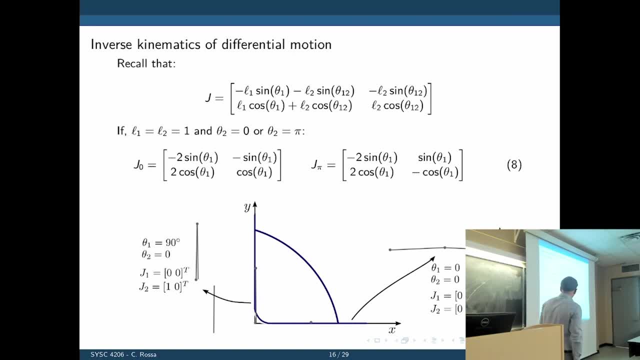 Theta 2,. excuse me, Theta 2 is zero, theta 2 is pi. So when the robot is here it's just going up and down because it's tracking a point very near the origin here. then theta 1 is 90 degrees. 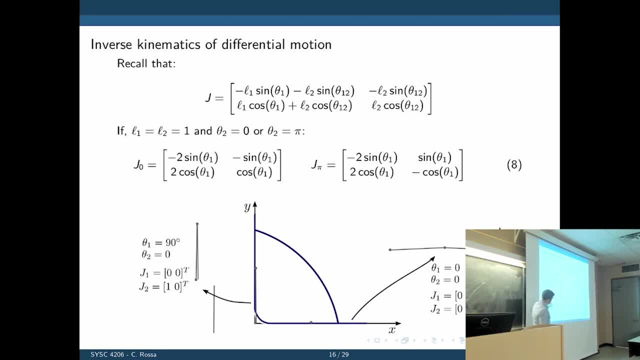 theta 2 should be 180.. This should be 180,, but anyways it does the same thing. We can see the resultant J1 and J2.. What can you tell from J2? That the only this one cannot create any direct any. 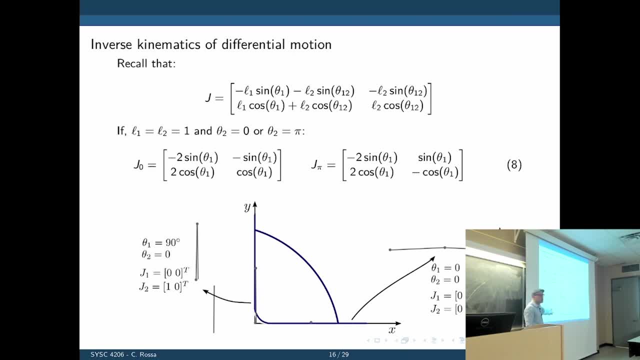 speed. This one can only create a speed in X, which it makes sense, because if the robot is going up and down, the tip can only move along X right, And if the robot is going fully stretched- it's now pointing that way- then theta 1 and theta 2 are: 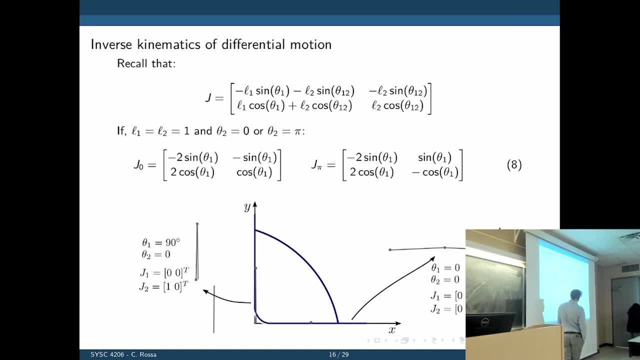 both zero. Look at what happens here. J1 and J2 are only in the Y direction. How do you explain the fact that a J1 is greater than J2? What is J1 doing? again, It's relating the speed of theta 1 to the speed of the tip. 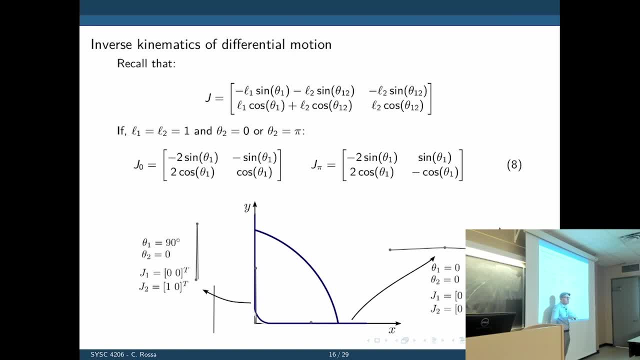 and J2 is the speed of theta 2 to the speed of the단 the tip. why is theta one then greater? because it has a bigger arm length. what's the idea? the speed there, isn't it? the radius times, the angular speed, right, so you? 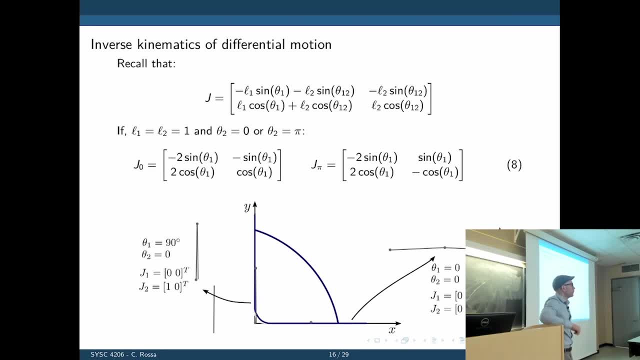 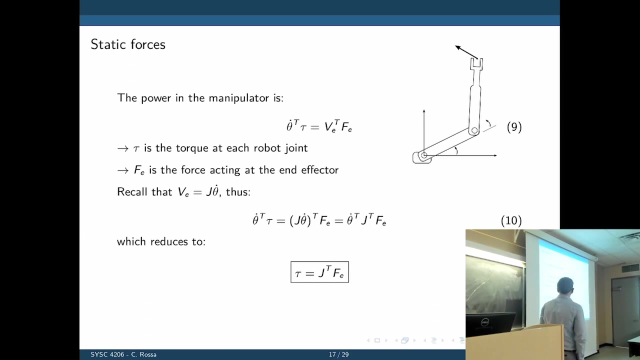 can see that these also depend clearly on the configuration of the robot and the structure of the room. okay, so this one just a type here. this should have been 180.. okay, one last thing. one last thing. we can use the same structure to now find the relation between torque and force. 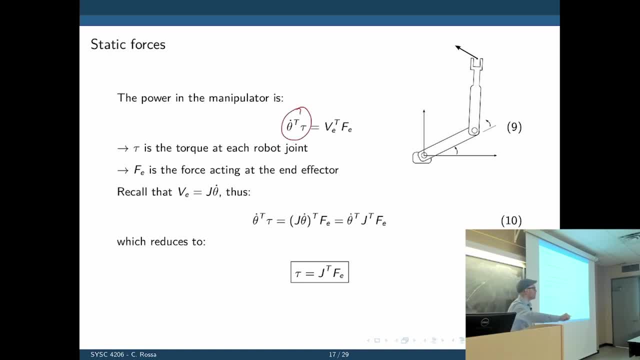 if you look at the cartesian, the joint space, we have a angular speed and they have a torque for each joint. so if you multiply them, if you multiply the speed of each joint with the torque of each joint, what you get the power in each joint. when i transpose the matrix like that, it means that 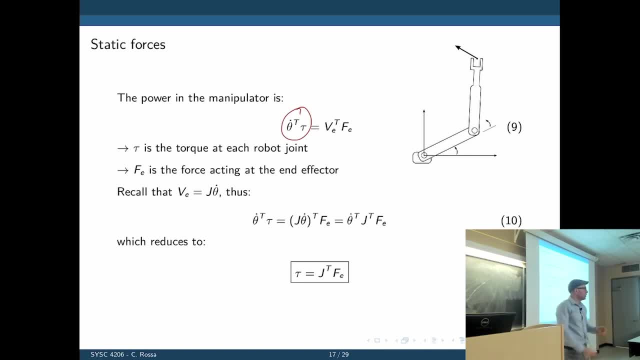 we're going to eventually just add everything up. right, it's going to be a row matrix times a column matrix. so you're basically doing theta one, dot, tau one, theta two, dots, tau, two, and so on, and then adding everything up. so that's the total power in the joint space. what happens in the cartesian space? well, it's the same, because now 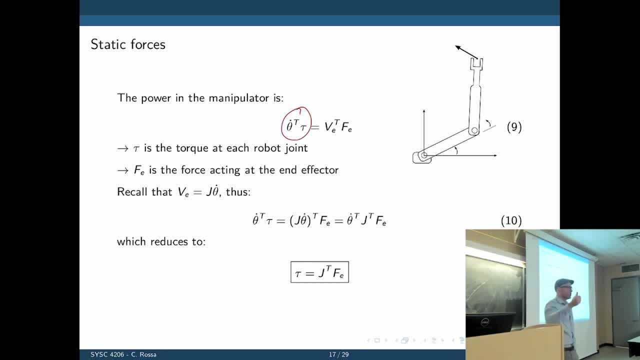 instead of torque we have a force developed at the tip, and instead of the angular position speed, we have the linear position of the tip v, e or the end factor. okay, so now we can establish this relation here: the torque in the joint space equal to the torque. 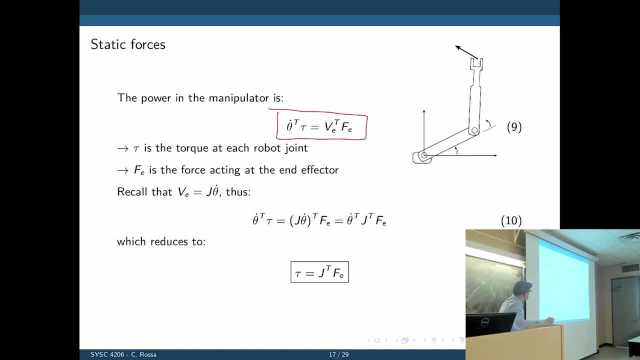 excuse me, the power in joint space equals to the power in cartesian space. we had an expression for v that are, and you can relate v to theta. how do we do that? v is with respect to theta dot. is j theta dot, isn't it? it's j theta dot, yeah. 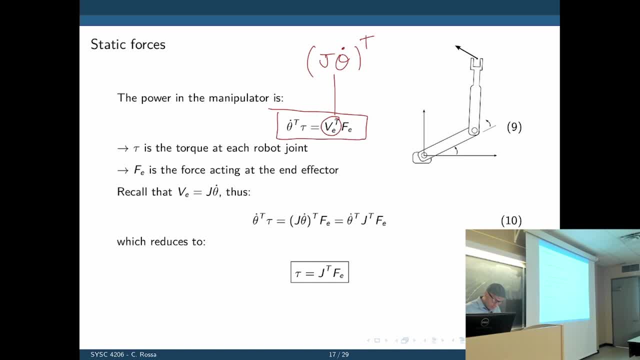 so the transpose. okay, let me do this in one step at a time. so i'm replacing the speed with j theta dot, so now i can relate this, expand this expression and then have j theta dot. all transposed times f, e. the transposed of a multiplication is the same as the multiplication of the transposed. 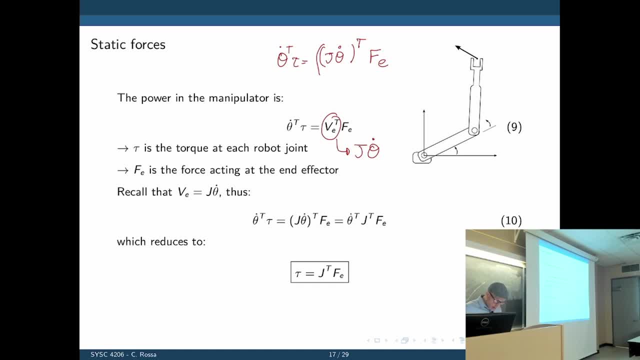 so this theta, this transpose, can go on theta and on j instead, which means that i can now cancel these two out and you have. the torque equals to the transposed of the jacobian times. the force: interesting. so the jacobian itself relates speed. the transpose of the jacobian gives the relation between: 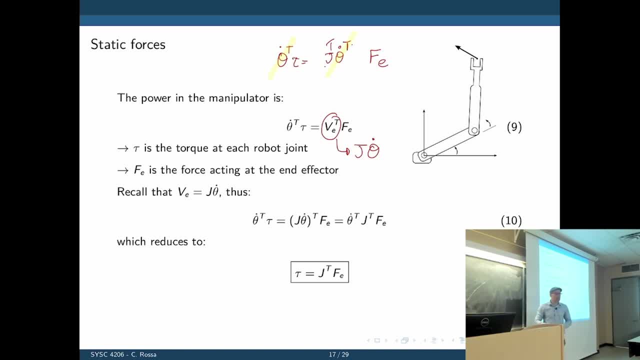 torque in each joint and the force exerted by the robot at the end effect. so, uh, the force acting on the end effector means that the force is acting on the end effector, mean that the robot is acting a force, for example, on the knee right. 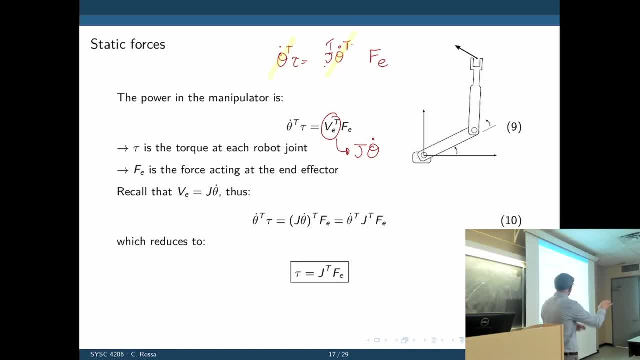 Yes, This is the force, Let's say the static force. So if you position the robot like that and you just apply torque to each of the robot, it will apply force to your hand. That can be calculated through that, The transposed of the Jacobi. 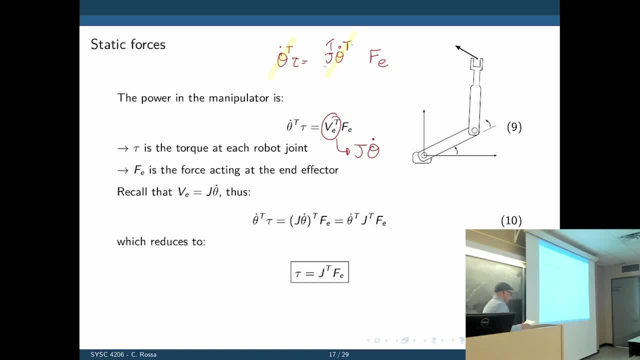 Okay, Any questions? No, But once again remember, always remember, that the Jacobian here changes constantly as soon as the robot changes position, because it's a direct function of theta 1. And theta 2 for that particular configuration, for that particular robot. 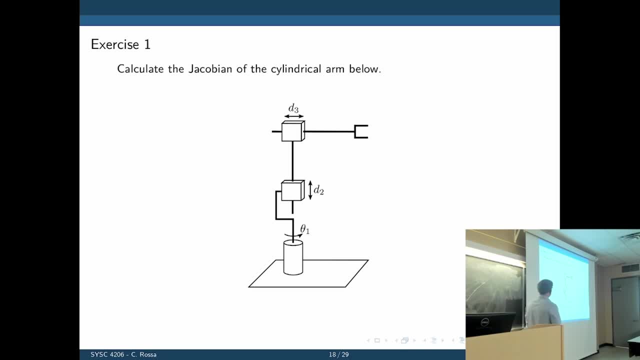 Okay, So if there are no questions, let's do two exercises, three, if we have time. First one: calculate the Jacobian of the cylindrical arm below. So calculate the Jacobian of the cylindrical arm below. Go ahead. What did you do first? 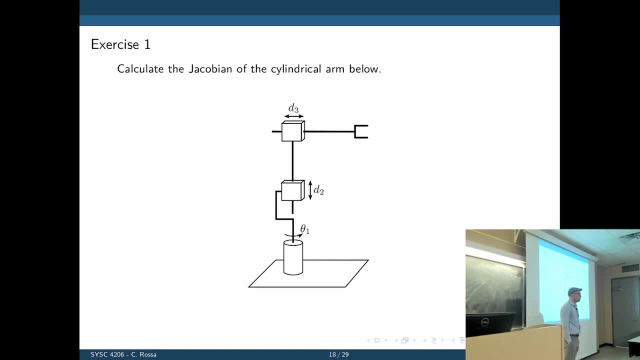 Find the forward kinematics. So we need the how many degrees of freedom we have here. We have three, Three right Three Cartesian positions, So we need to determine the expression for X, Y and Z, Then how many actuation points we have. 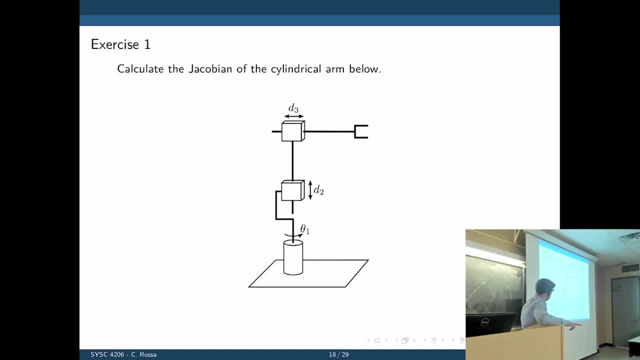 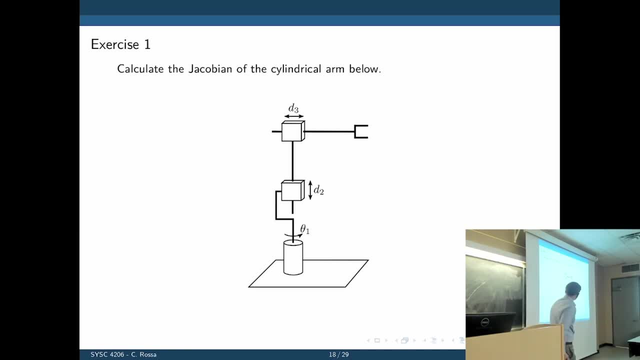 So what's the size of the Jacobian? It's a three-by-three matrix. Okay, I'm going to spare you the trouble of finding the forward kinematics, because that was covered in a past lecture. All right, So here is the homogenous transformation matrix, if you want to practice frame assignments. 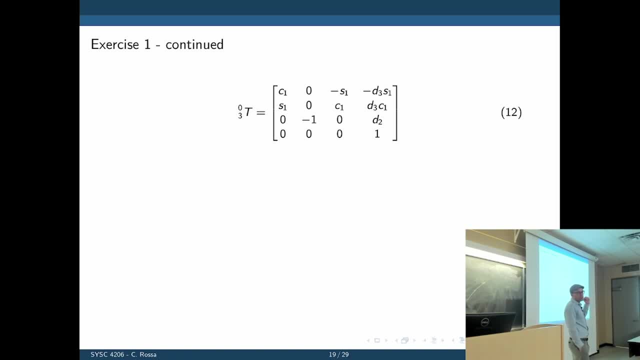 and forward kinematics. you can try to get here on your own later. But that's the homogenous transformation from frame 3 to 0.. Where is x, y and z? There, That's the vector: y, x, y and z. So the x position of the tooltip is negative. d3: sine of 1.. 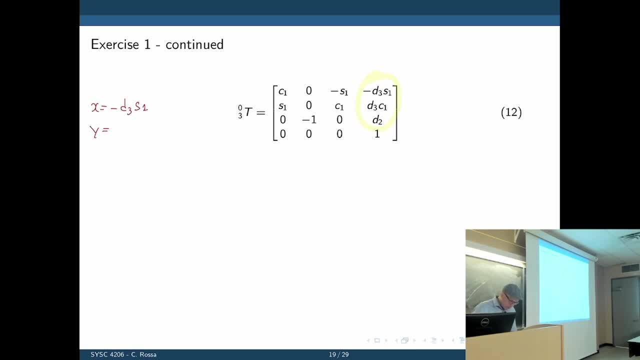 The y position of the tooltip is d3, cosine of 1, and the z position is d2.. What is the Jacobian? Let's just define Jacobian Is the partial derivative. what's the first row of x with respect to theta 1, then the partial derivative. 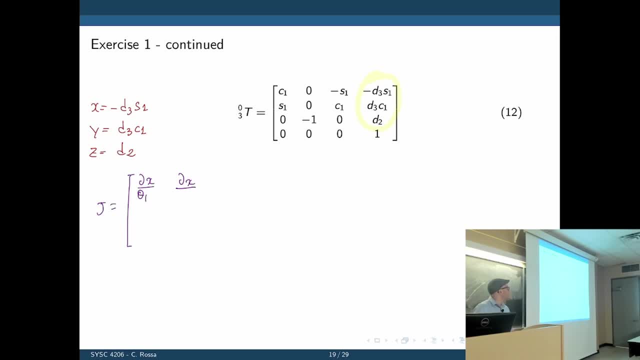 of x with respect to hold on, there's no thing. 2 to what? now? d2 and the partial derivative of X with respect to d3.. Sorry, d2, d3.. Very good, What's the second row? It's the same, but now with respect to. 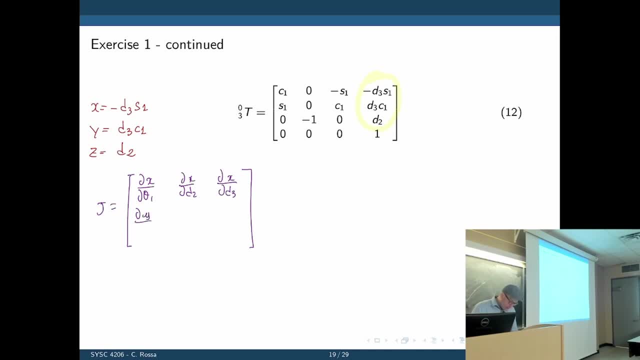 d2.. What is the derivative of Y? And then, lastly, the derivative of Y, excuse me- Z, with respect to theta1,, with respect to theta2, and with respect to- oh sorry, I made the same mistake now- Theta d2, d3.. 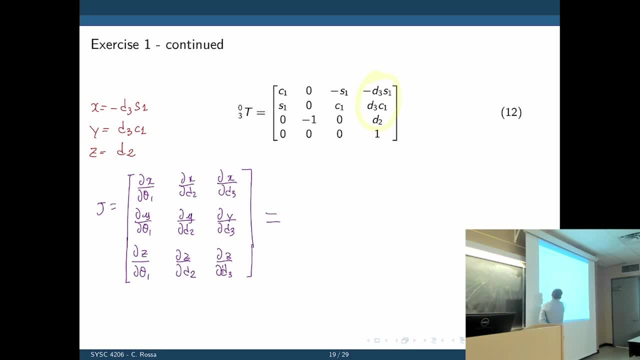 Okay, so again, first degree of freedom, partial derivatives of all actuation variables. second and third. So what is the first row? What's the partial derivative of X with respect to theta1?? Theta1 is sine, becomes cosine, so it's negative d3 cosine of 1.. 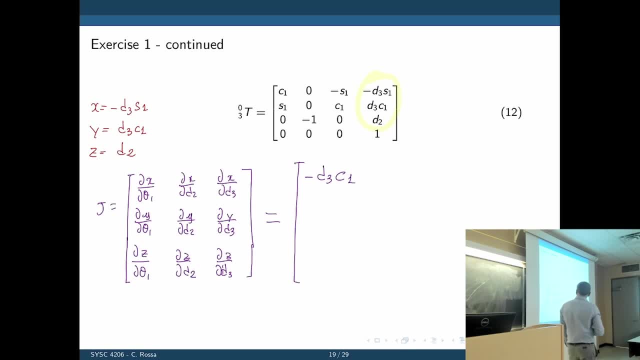 What's the second element? Partial derivative of X with respect to d2.. What is that? Partial derivative of X with respect to d2.. Zero, Zero. What is that saying It's? the partial derivative of X with respect to d2 is zero. 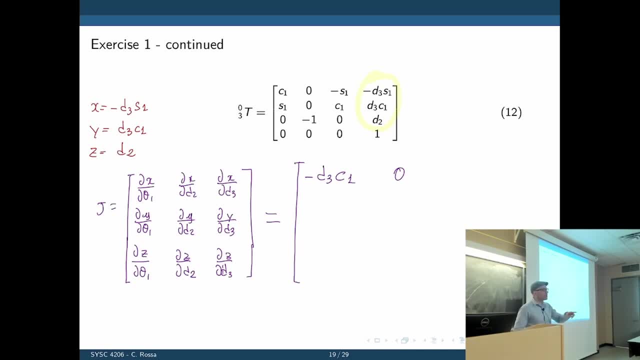 So that means that a d2 cannot affect X? Very good, D2 cannot affect X. Is that the case? Yes, because d2 only controls the vertical position, Which here is Z. All right, Z, let's put a X and Y. 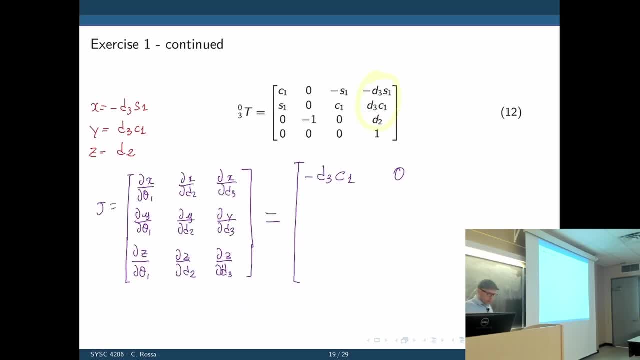 I like that. What's the last one? The partial derivative of X with respect to d3 is minus sine of 1.. Second row: partial derivative of Y with respect to theta1 is d3 sine of 1.. Cosine is negative sine right. 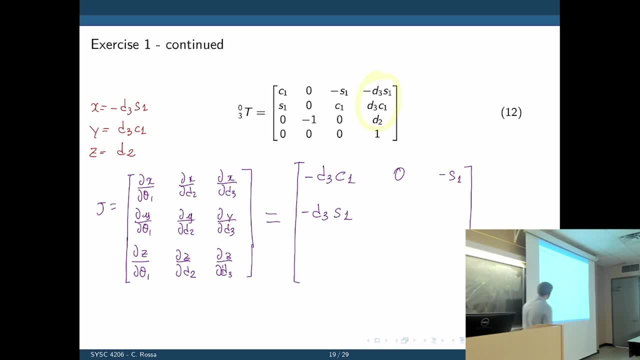 Negative d3 sine of 1.. What is coming next? D, partial derivative of Y, d2.. What is that? Zero, Zero Again. d2 cannot affect Y, Y can only affect Z. so that makes sense to be zero. 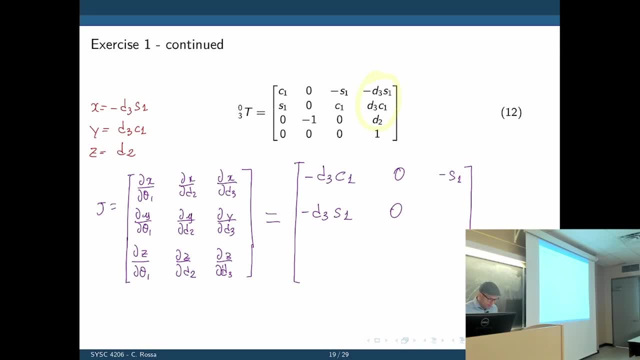 And then the last term is partial derivative of Y with respect to d, which is d3,, which is C1.. Last row, all partial derivatives with respect to of Z. Now, what is partial derivative of Z with respect to theta1?? 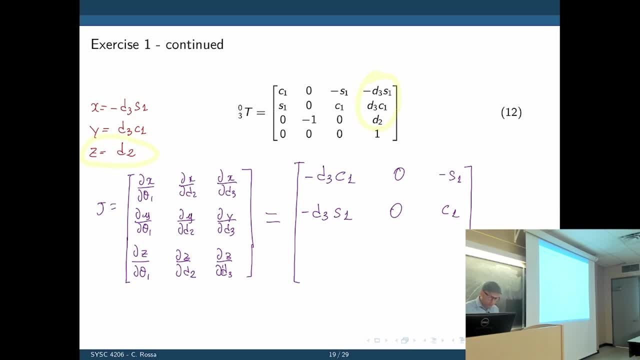 Come on, folks, wake up. Partial derivative of Z with respect to theta1? Zero, Zero. with respect to d2? One One And with respect To d3? Zero. So this is saying that d2 cannot affect. 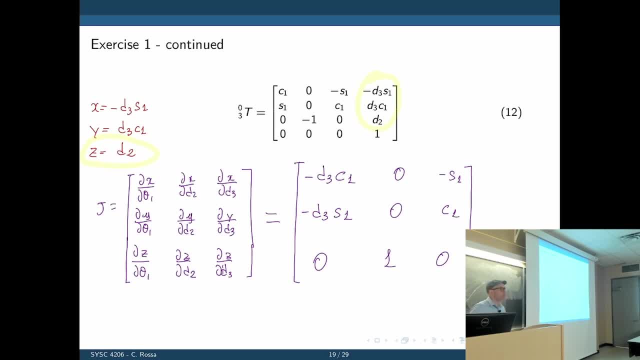 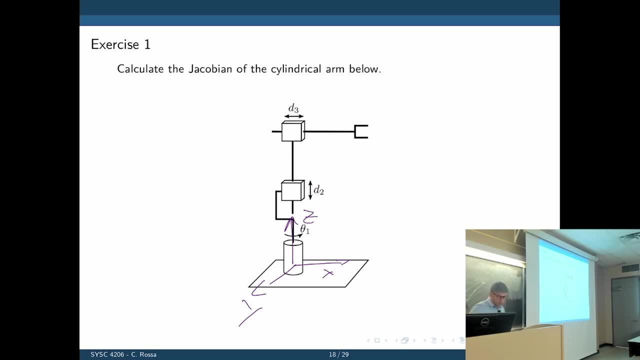 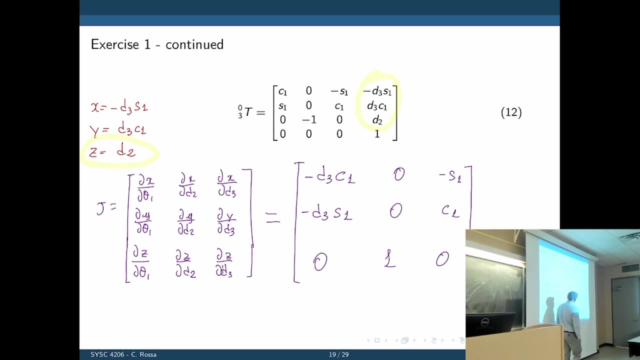 cannot be affected by theta1 or d3.. And that's exactly what it is, because it only controls the Z position. Okay, and that's the Jacobian. Is that right? Yeah, Okay, All right. So this problem doesn't ask, but let's find the singular configuration. 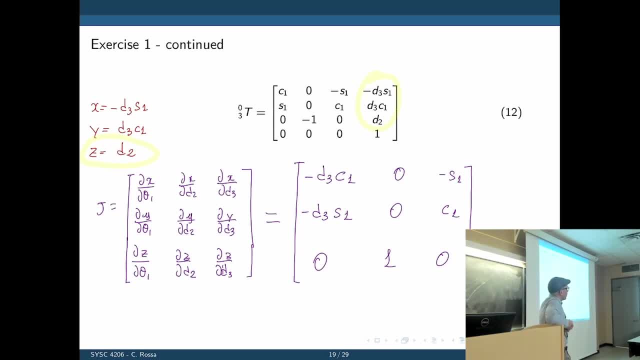 What's the singularity of this robot arm? We need to find the determinant, So I'm going to take the Jacobian. we calculated here. I think there was actually exercise four. that asks for the singularity, So let's move to exercise. 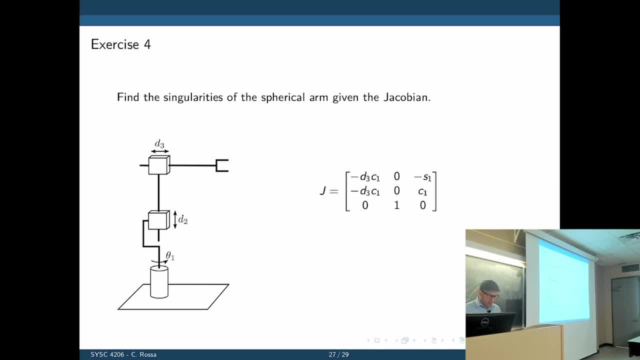 four. Yeah, that's the Jacobian we just found, isn't it? Yeah? and then let's try to find the singularity, which means the determinant of J. How do you find the determinant of a three by three? I don't know how you learned it. 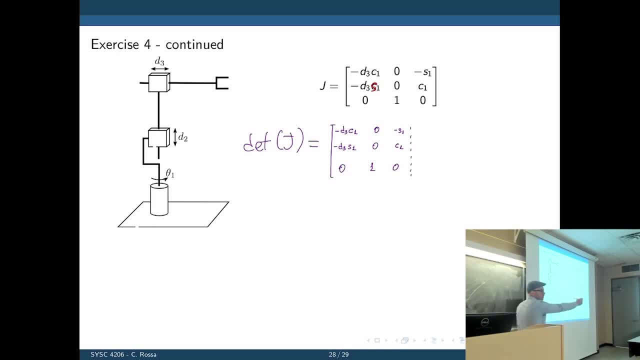 but I learned it to copy the first two rows over: Yeah, And now we can find the determinant by multiplying that which is 0,, multiplying this, which is also 0, and multiplying that which is negative. d3 sine of 1. 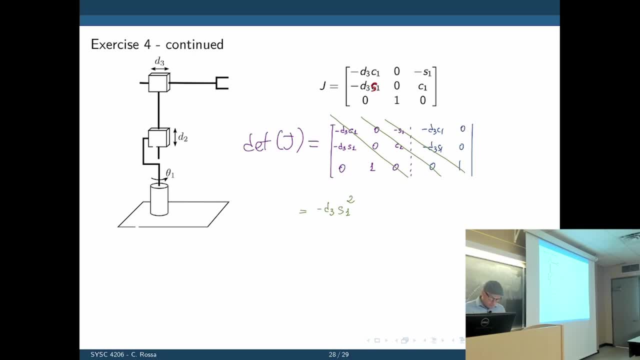 squared, Then minus that 0,, minus this, which is plus sorry, this is positive- plus d3 cosine of 1 squared plus 0. Does that make sense? Yeah, Let me do a color here that you can actually read There: What can you do You? 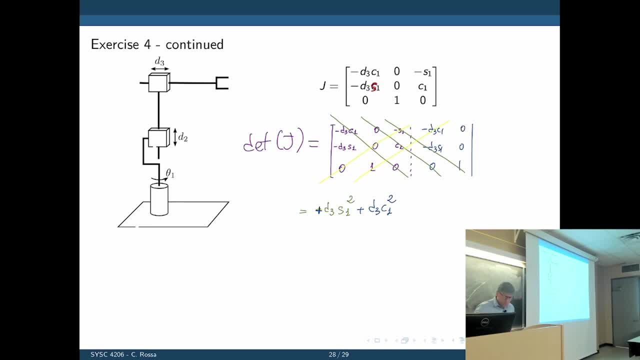 can simplify that right. If you factor out d3, we have s1 squared plus cosine 1 squared, and that is, That is d3.. So the determinant of J is d3.. How do we make that zero? 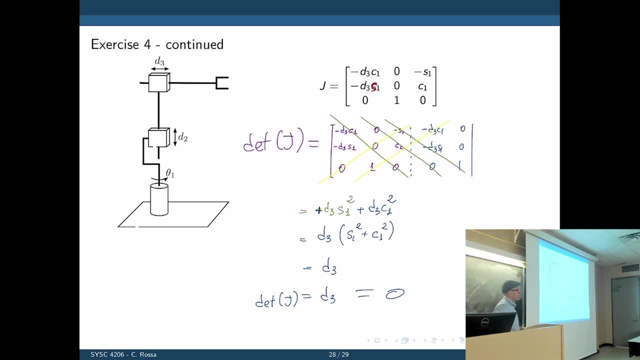 Just equate that to zero. Yeah, If we equate that to zero, how is that steps? oh, photousecond. Yeah, who das to? punches Sam at a singularity. You can only rotate like that. You cannot create speed in any other direction. 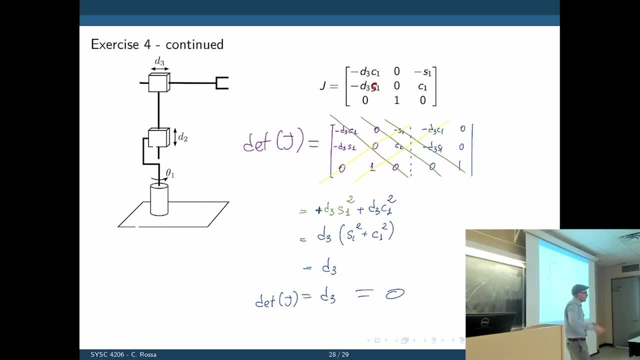 because we lost the arm length to do rotations like that. Okay, So you wouldn't be able, in other words, you wouldn't be able- to produce a speed in which directions X or Y, You'll only be able to control it. 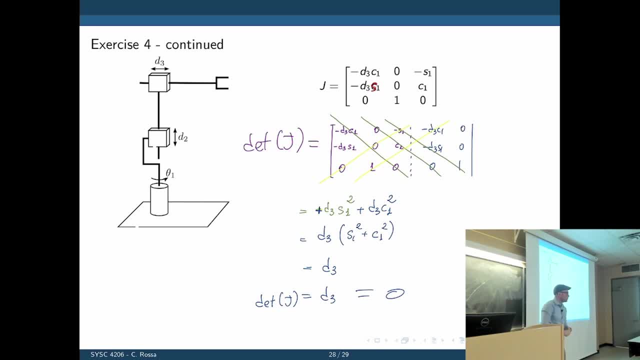 the rotation speed, like that, and then the up and down Z speed. Yeah, So the singular configuration requires D3 to be zero, So this goes away, And we are now in a point there. Alright, so how do we now make the robot move in X and Y direction? 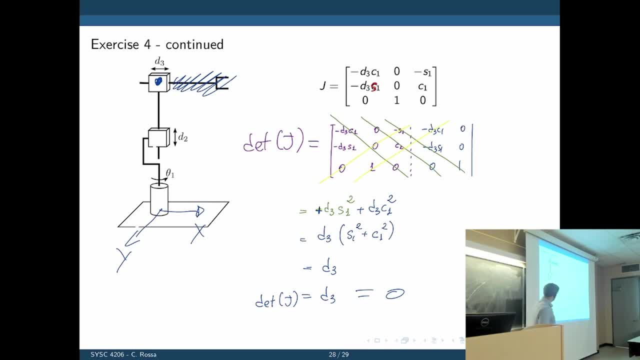 We can't, Because the only way we could do that is if we had an arm length and then the base would rotate Like that. But that's gone, So they can only have a speed now in D Or a rotation speed. Yeah, we can still control D2.. 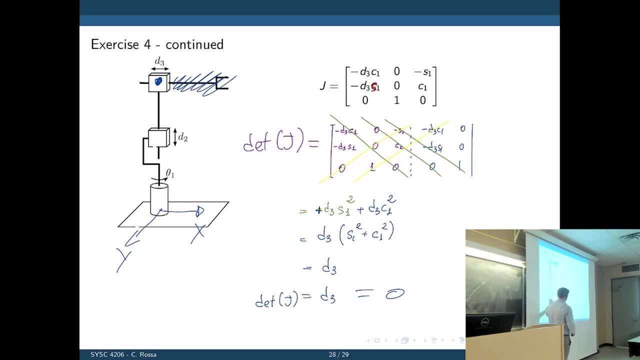 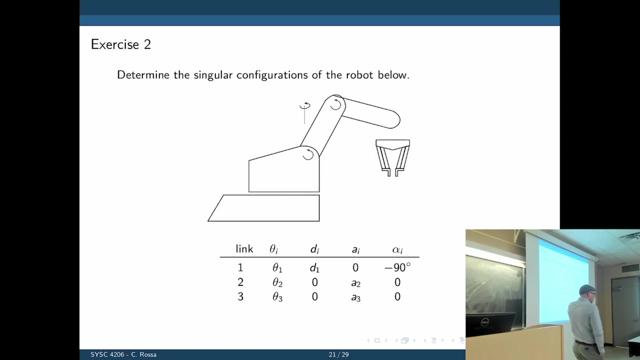 Alright, so D2 would create a speed in Z, But the speed in Y and X would be gone. So D3 is zero. Okay, let's do quickly one more here, Exercise 2.. It's not showing in my not displaying here, for some reason. 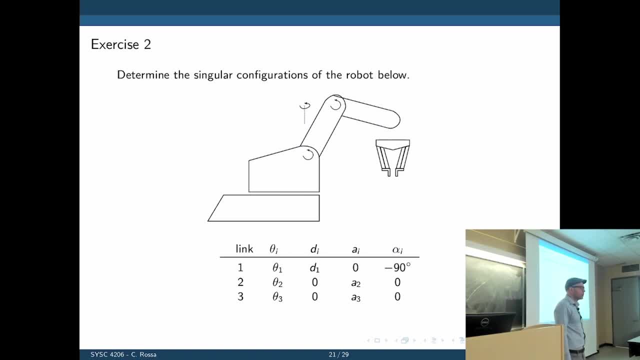 That's the app I'm using, But it should be shown more clearly in your copy. there We have a 3-DOF, 4-DOF, a 3-DOF robot arm. One, two, three Degrees of freedom. 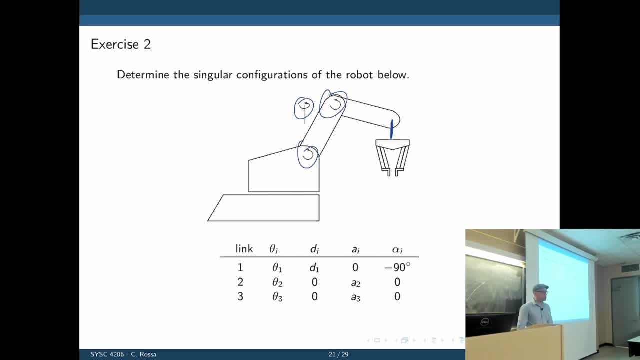 Those are the DH parameters. We want to find the singular configurations of that robot. So I'm giving you here the transformation matrix And the transformation matrix. this one has a typo. I don't know if I updated this In bright space. the last line is missing there. 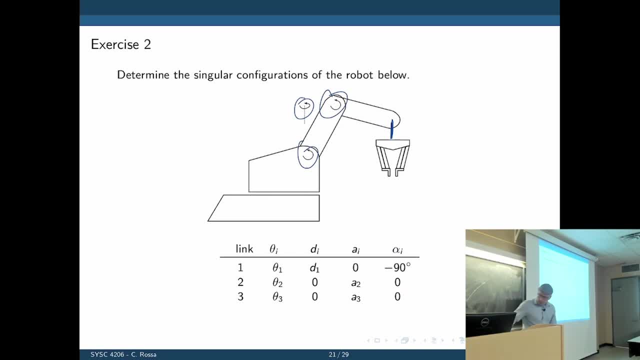 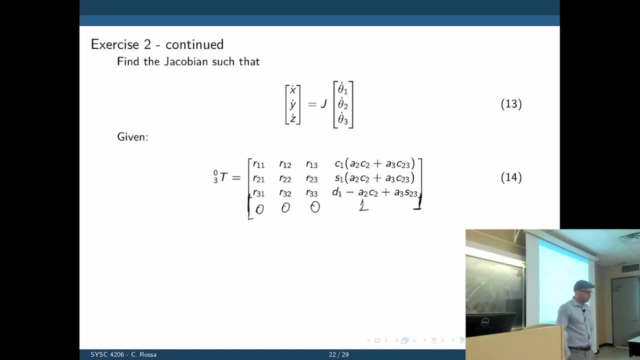 But it doesn't really matter, right? Oh, sorry, That one, The last row, is missing. Okay, so if you want to find the singular configuration, what's the first step? Forward kinematics, Forward kinematics, which is already given in 14.. 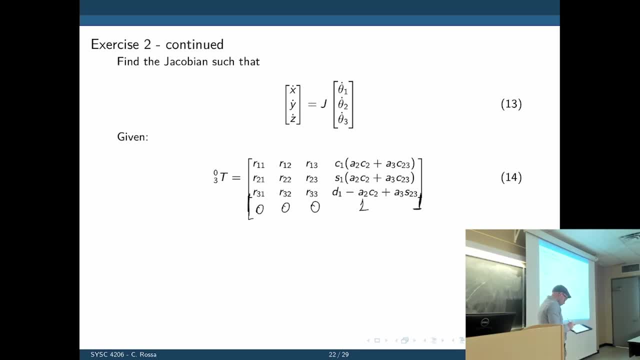 Then 2.. 2, the Jacobian. What is the Jacobian for this one, For this robot? How many degrees of freedom do we have X, Y and Z? How many control variables? Three, So we have a nine element Jacobian. 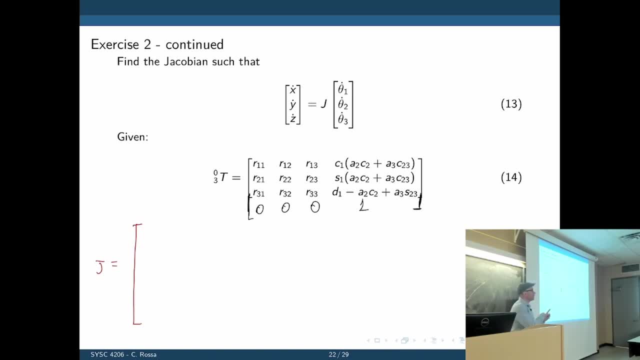 The first row is, let's say, X, Partial derivative with respect to theta 1,, 2, and 3.. So what's the first row? the first cell Partial derivative of X, which is right here, With respect to theta 1.. 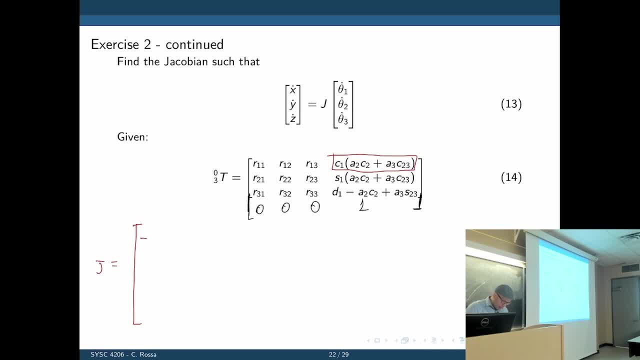 That is negative sine 1.. And everything else remains the same. Then the second element is the partial derivative of X, The partial derivative of X with respect to theta 2.. What is that? Cos 1 times A2, sine 2, negative. 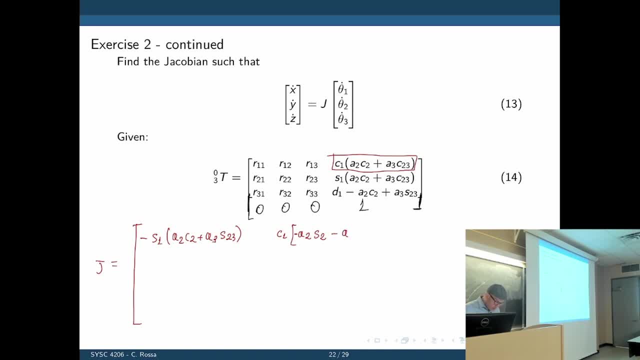 Plus or minus A3, sine of 2, 3.. And the last cell there is the partial derivative of X, Again in red, with respect to theta 3.. So the first one here is only the first element, is only a function of theta 2.. 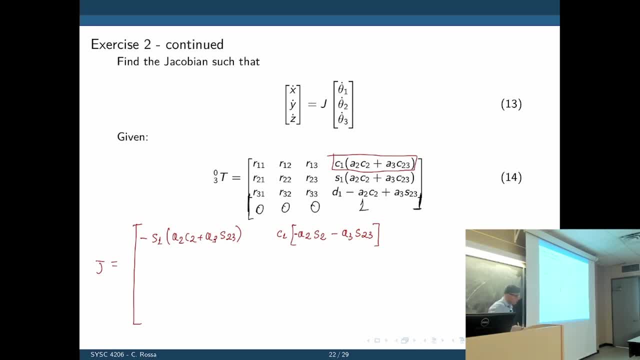 So that's zero. And then you are left with cosine 1 times A3.. Times A3. Times sine of 2, 3.. Negative: What is the second? one Second line is partial derivative of Y With respect to theta 1.. 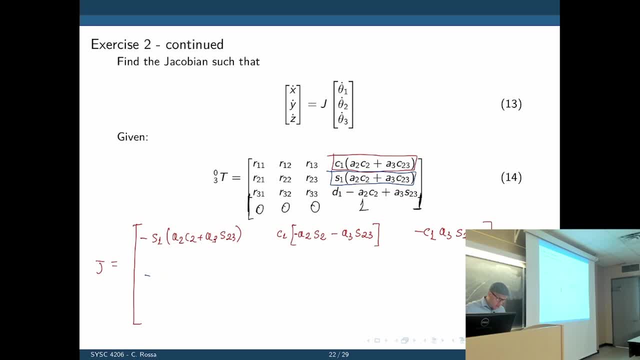 That is negative C1.. Sorry, no, that's just C1.. Cosine 1, A2, C2. Plus A2, 3, cosine 2, 3.. With respect to theta 2. Is S1, A2, cosine 2.? 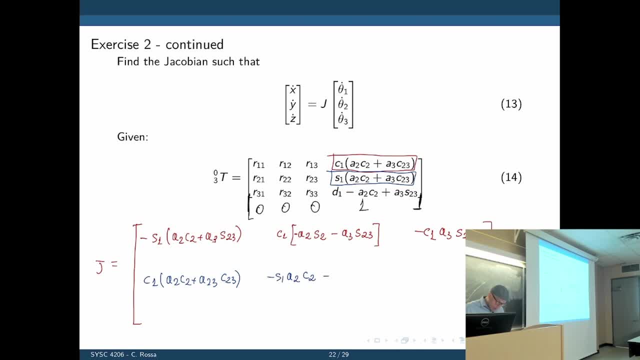 Negative Minus S1, A3,, sine 2, 3.. And then the last one is with respect to theta 3.. That is sine 1, A3,, sine 2, 3.. Negative, Yeah, Sort of. 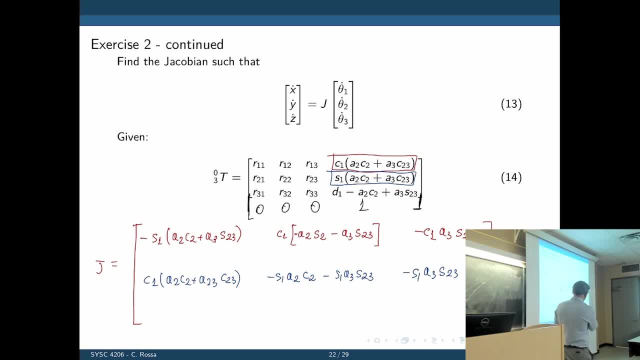 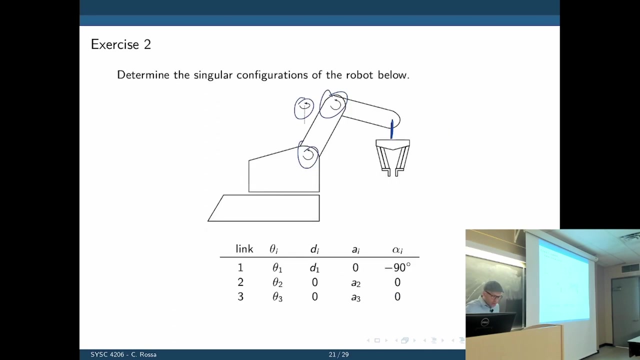 Does that make sense? So what's the last one? See, if you follow. Last one is Z with respect to theta 1, which is What's the partial derivative, Zero. Zero, That means joint 1 cannot affect Z. Is that the case for this robot? 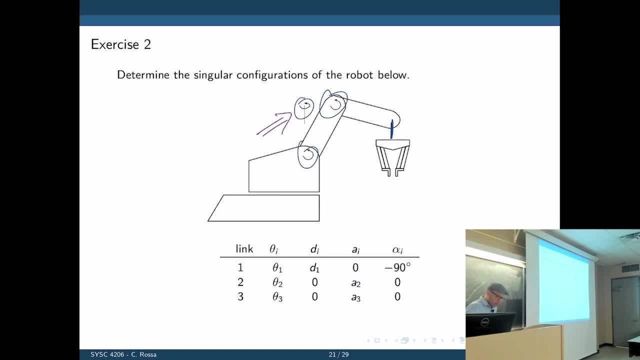 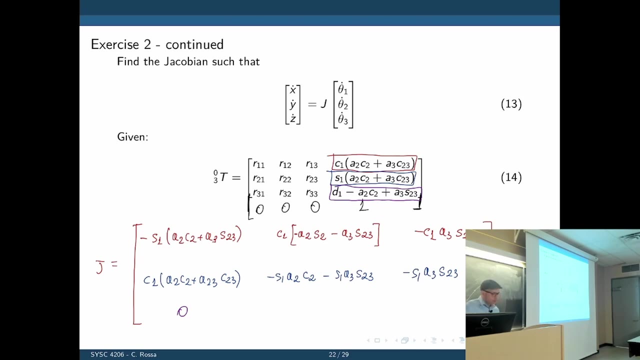 Joint 1 cannot affect Z. Yeah, Then the next one is Z with respect to theta 2. is What is that Z with respect to theta 2.. Z with respect to theta 2.. Cosine of 2 becomes negative sine of 2.. 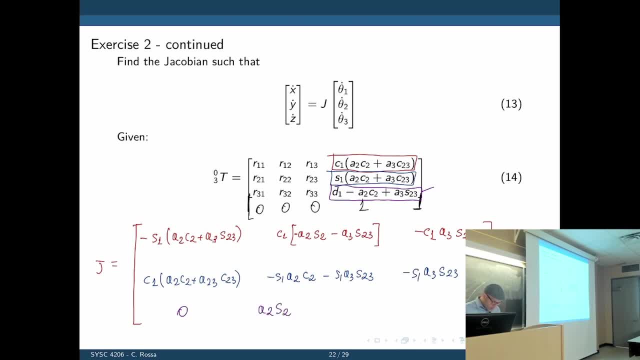 So A2, sine of 2.. Plus A3, cosine 2, 3.. And then the last one is that, with respect to Z, Excuse me- To theta 3.. That is A3, cosine 2, 3.. 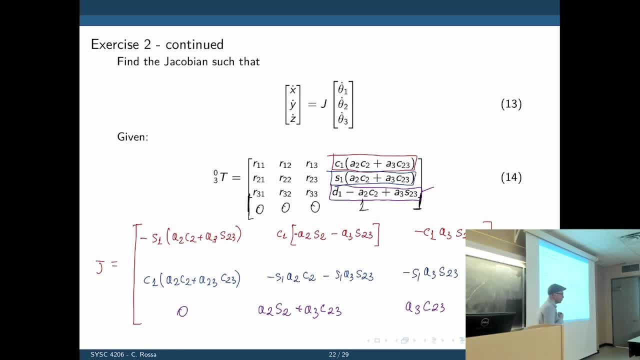 That's the Jacobian. What do we do next? once we found the Jacobian, We find the determinant. Now the determinant of this Jacobian has around 1,, 2,, 3, 9. There's around 50 elements in it. 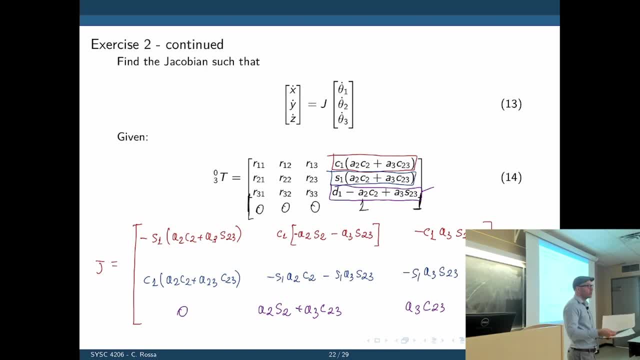 If you multiply everything out, Of course, you don't have time to do that In the middle one. is that supposed to be minus S1, A2, S2?? This one, No. from the left side, This To the right. 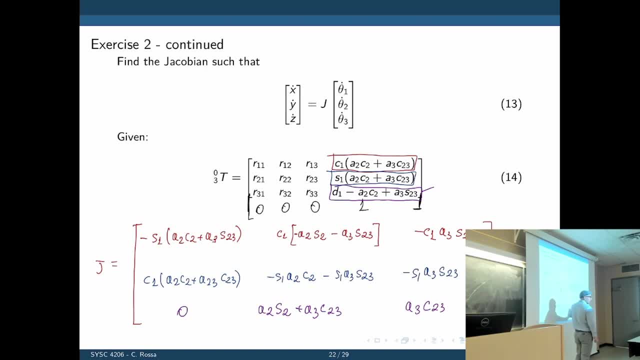 That one. No, no, Oh, my god, Make a decision. Miles The middle, Yeah, here's the middle. Yeah, minus S1, A2.. That's supposed to be S2.. That is the derivative of this with respect to theta 2.. 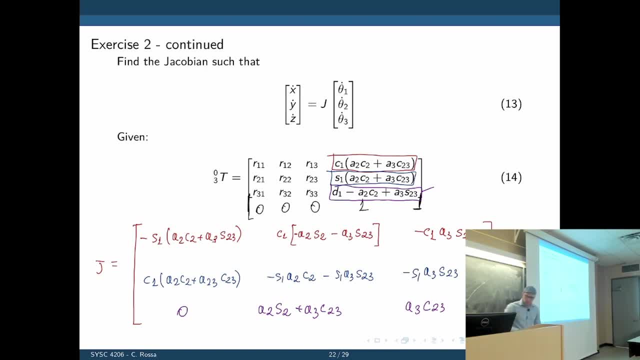 So, should it be Yes, Should it be Yeah, S2. Very good, Okay, so I'm not going to do the determinant of this, because this is giant and then you have to simplify. I can post that in the solution later, but after simplification, let the magic happen. 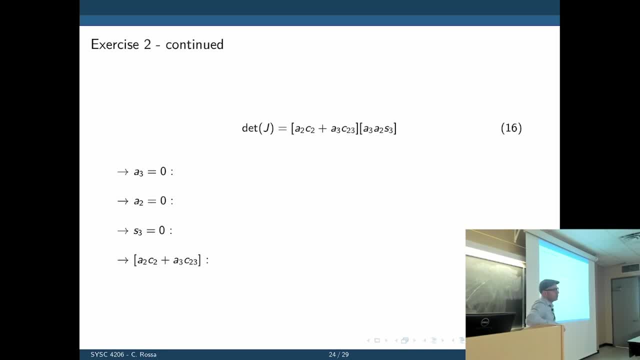 and that's the determinant. Would we have to make the magic Not with a three by three matrix? Two by two, Two by two, potentially Not six by six? What about the determinant of one by one? Can you do that one? 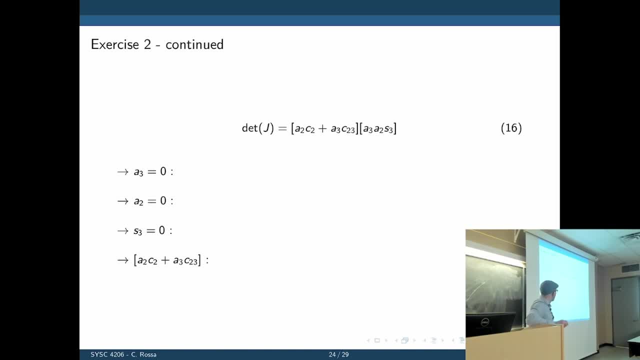 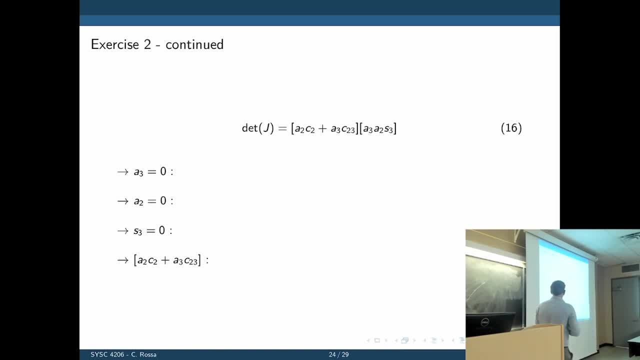 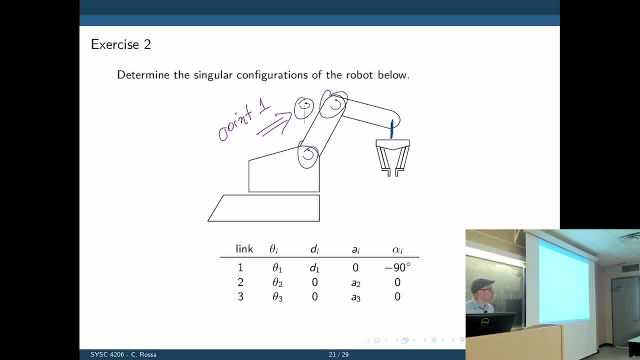 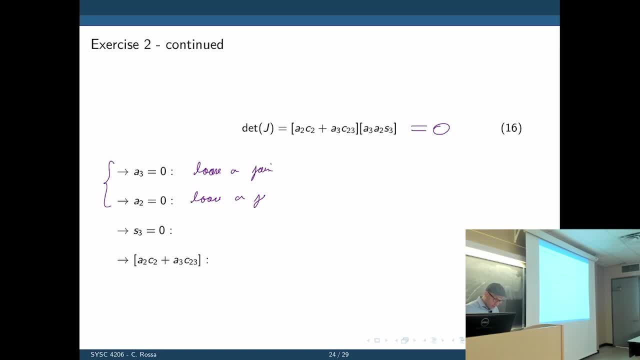 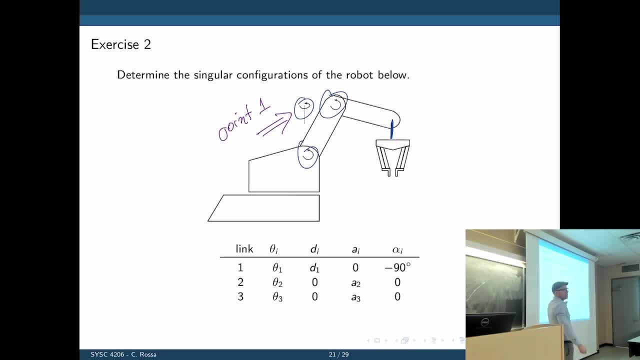 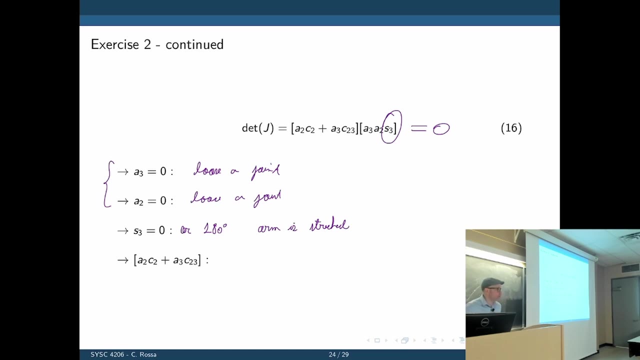 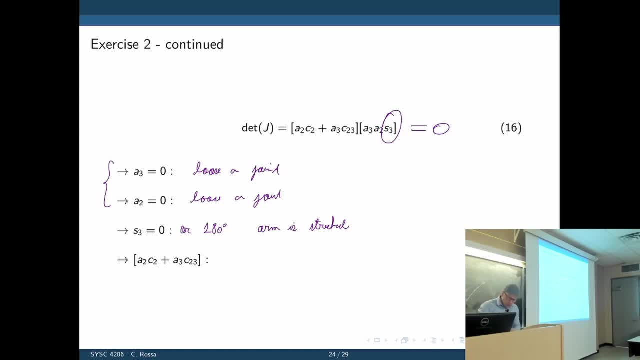 So what does that mean physically If you look at the robot? let's look at the robot here. What is? this is theta two, this is theta three, this is A2, this is A3.. This is our x-axis, y and z. 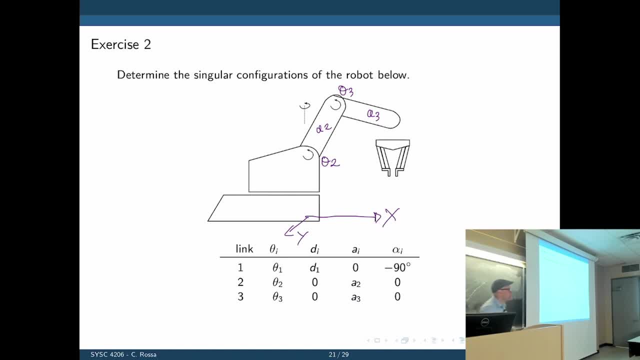 So what is A2 cosine of theta two Is the projection of arm two on x. A2 cosine of theta two is the projection of arm two on x. Is that clear? A3 cosine of theta two plus theta three is the projection of arm three. 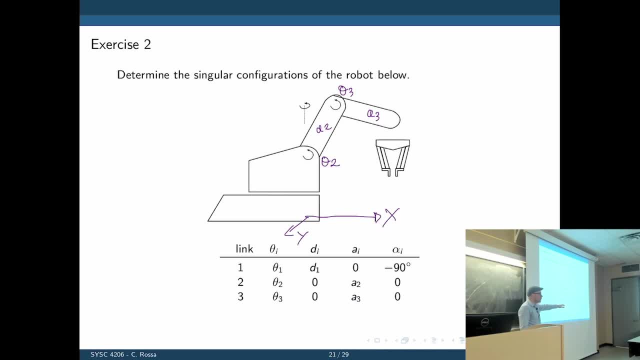 on the x-axis. So when you have A2 cosine of two plus A3 cosine of two, three equals to zero. what you are saying is: I want the projection of both arms, two and three, on x to be zero. In which configuration is the robot?